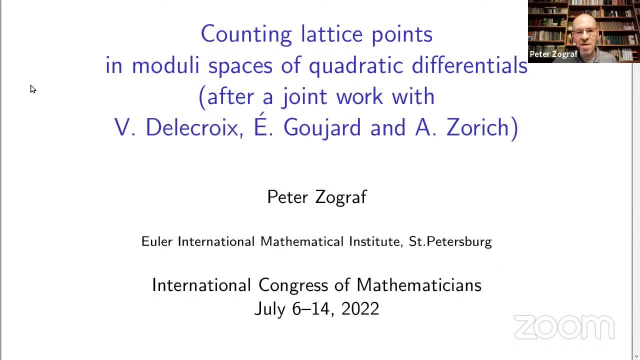 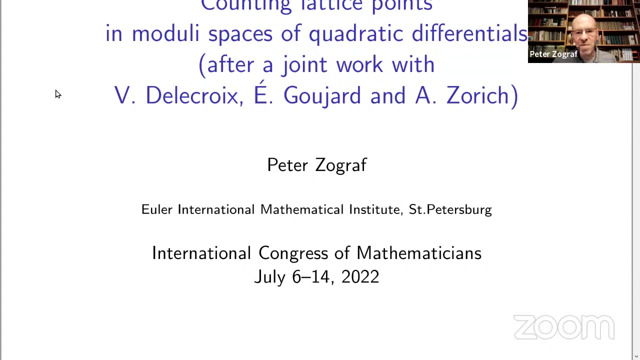 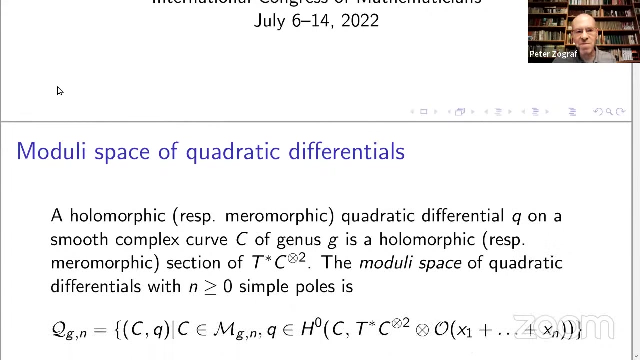 Another mention I found important is a nice work of Paul Norbury relating lattice points count in the modular space of curves to the intersection theory of the modular space. His results were rather important for us. So to begin with let me remind some basic facts about modular spaces of quadratic differentials. 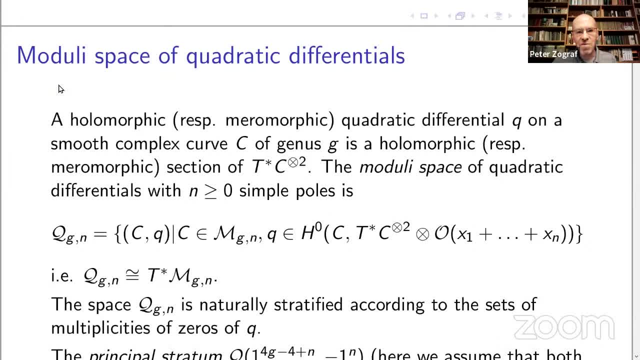 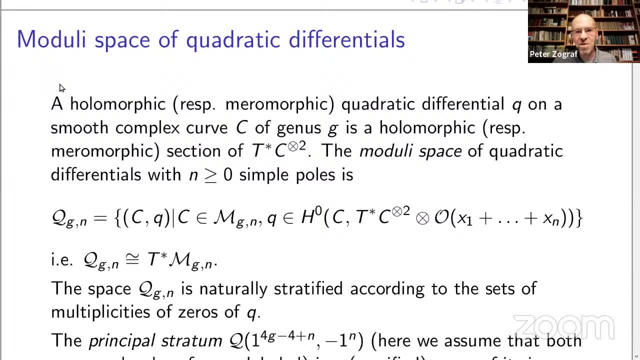 Holomorphic or meromorphic quadratic differences or meromorphic quadratic differential cube on the smooth, complex curve C of genus G is a holomorphic or meromorphic section of the square of the cotangent bundle to C, The modular space of quadratic differentials, with n simple poles. 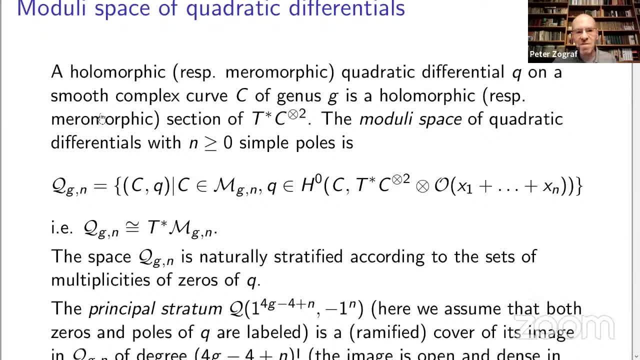 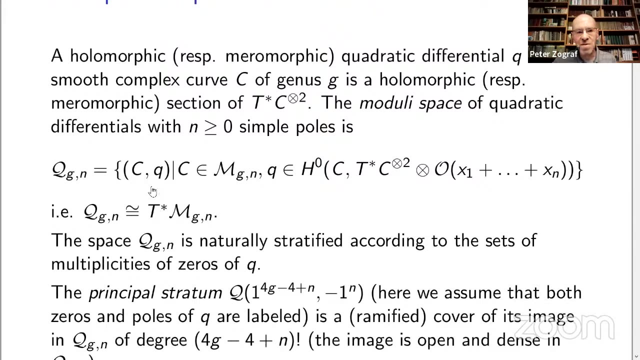 is this space of equivalent, of isomorphism, Classes of pairs, the complex curve C and the holomorphic section of the square, of the cotangent bundle twisted by the divisor of the marked points, In other words, the modular space of quadratic differentials. 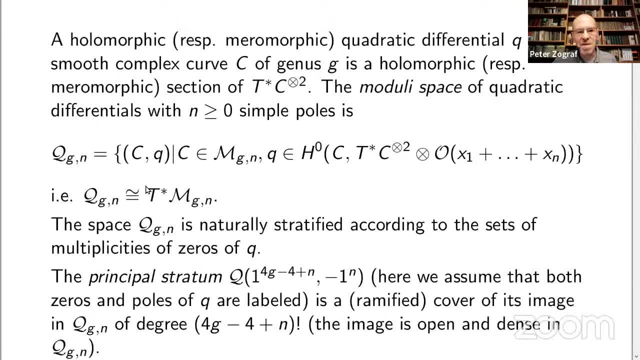 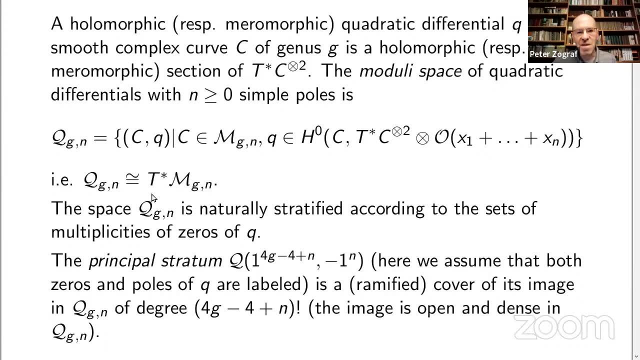 of genus G with n simple poles is isomorphic to the holomorphic cotangent bundle to the modular space of curves of genus G, curves with n marked points. The space Q is naturally stratified according to the sets of multiplicities of zeros of Q. 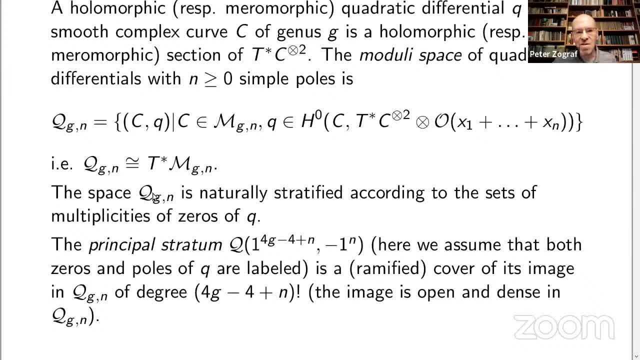 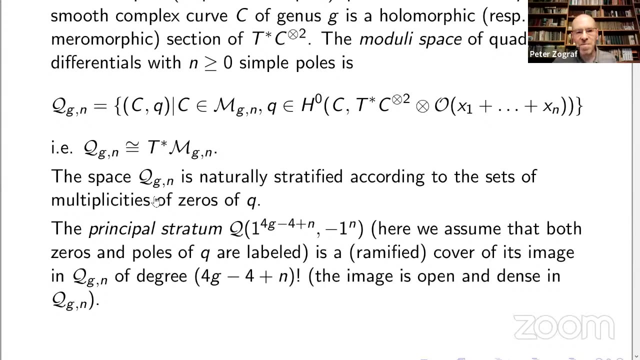 A generic situation is when all zeros are simple. There are four G minus four plus n, simple zeros on a curve, and we denote by Q of such a notation Here one to the four G minus four plus n is the number of zeros and minus one to the n. 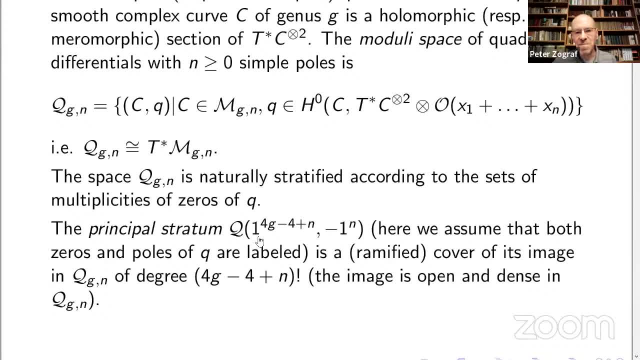 is the number of simple poles. We assume that both zeros and poles of Q are labeled, and then the principal stratum is a ramified cover of its image in the modular space Q of degree four, G minus four plus n, factorial, and the image is open and dense. 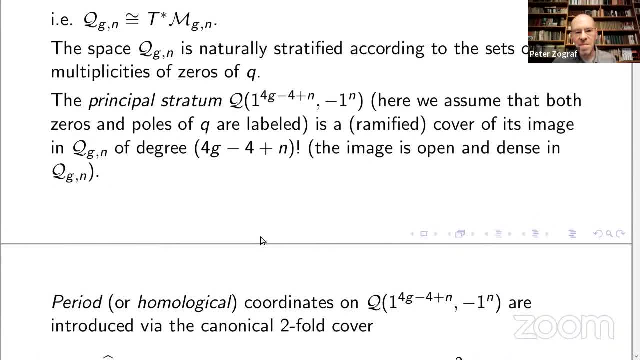 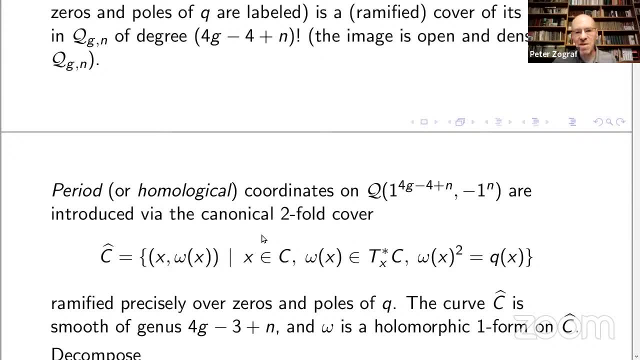 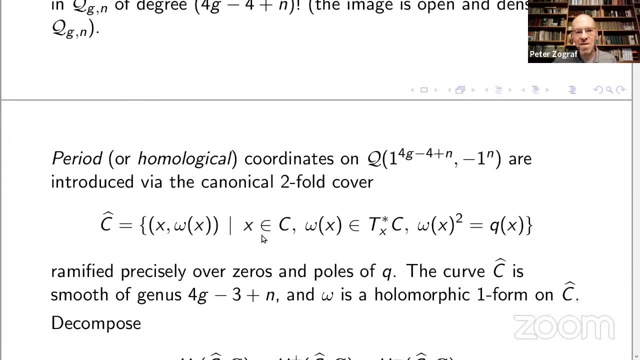 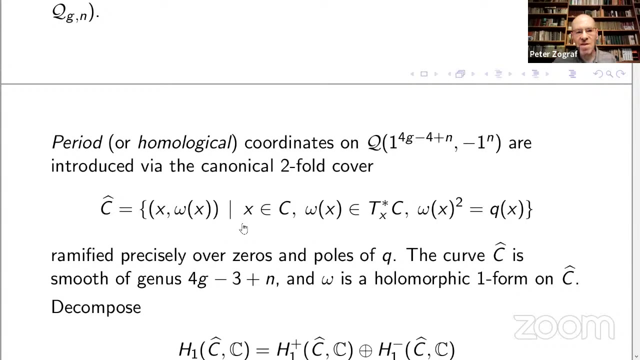 in Q. So we want now to introduce coordinates on the model on the principal stratum in the modular space of quadratic differentials. It is done via a canonical twofold cover, That is a curve C hat that lives in the cotangent bundle to C. 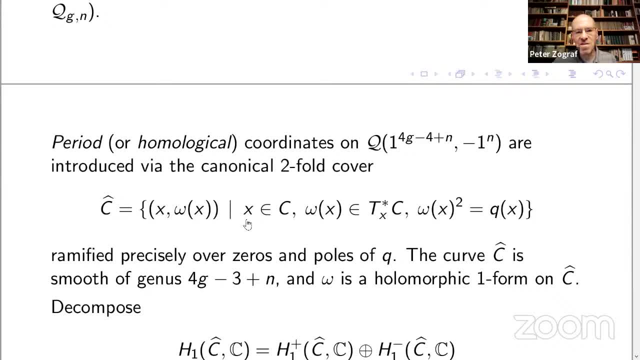 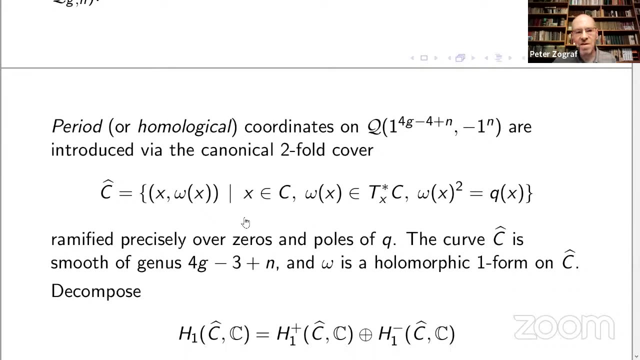 And here you see, X is a point in C and omega of X is a covector such that its square is the quadratic differential. This cover, that's a twofold cover that is ramified precisely over zeros and poles of Q, Over zeros, omega has. 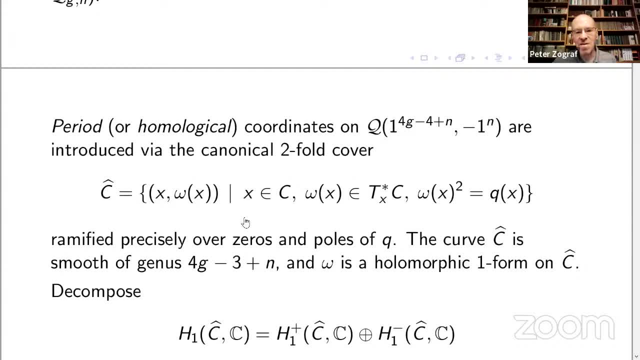 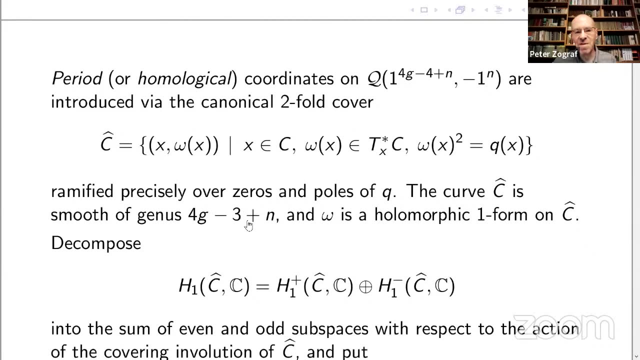 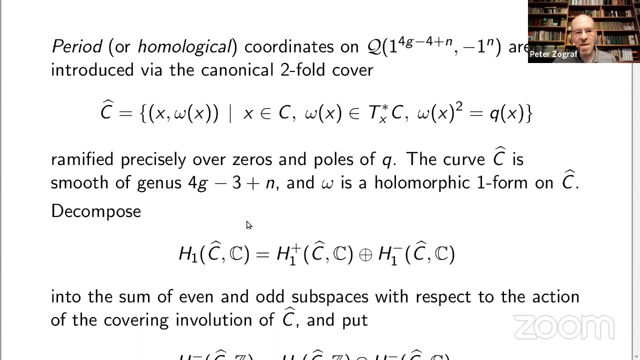 double zeros and its regular at the inverse images of pole of Q. The curve C hat is smooth of genus four, G minus three plus n, and omega is a holomorphic planform on C. Let us decompose the first homology group of C hat. 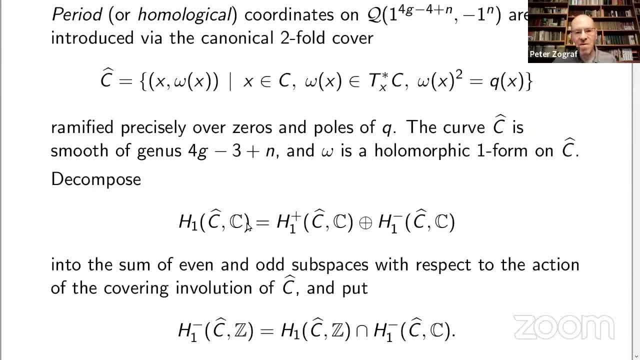 with complex coefficients into the sum of eigen spaces of the covering involution, H one plus and H one minus, where H one plus is the subspace, even subspace and H one minus is an odd subspace. in H one homology of C with complex coefficients. 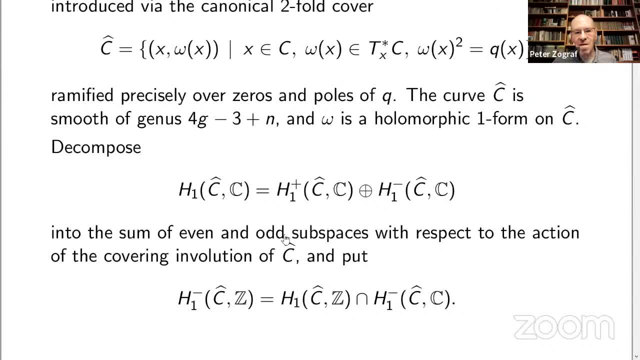 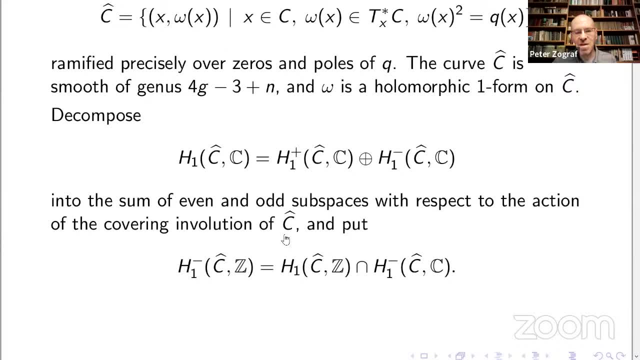 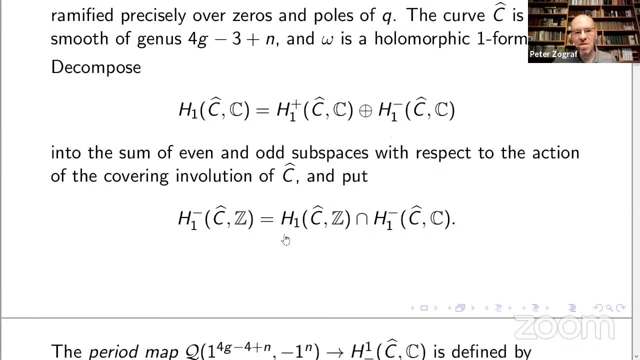 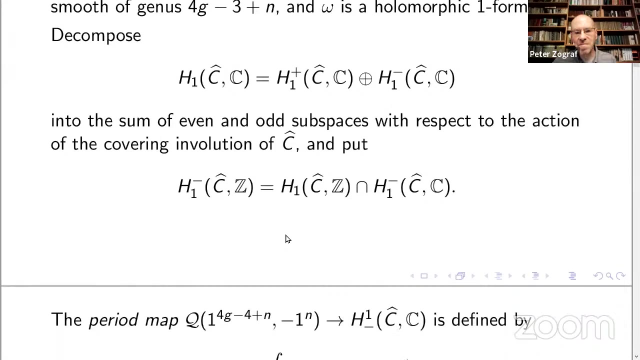 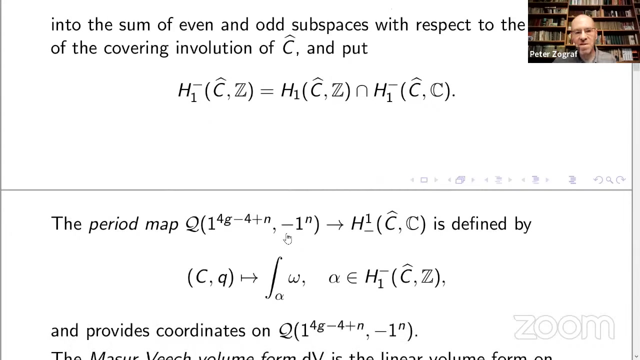 Let us now put H, one with superscript minus, to be the group of odd homology classes on C hat. The period map is a map from the principle stratum in the modular space of quadratic differentials to the odd cohomology group of C hat. 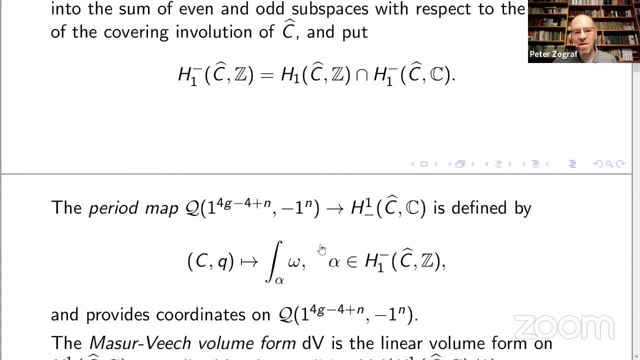 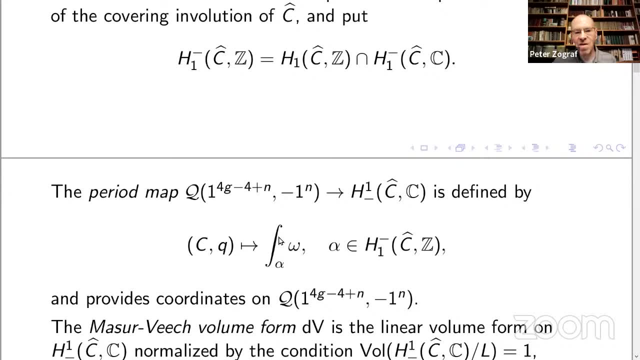 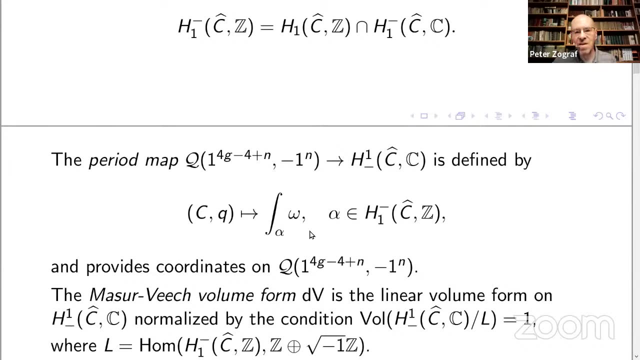 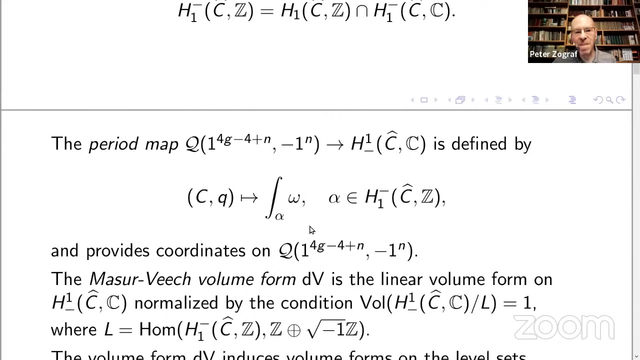 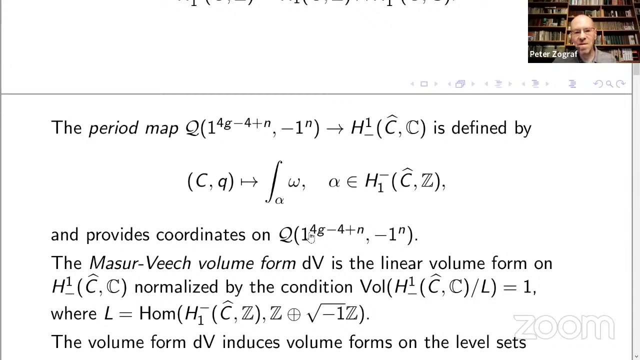 with coefficients in C is defined by the following formula: That's for the pair CQ, That's the integral over the odd homology classes of C hat of the quadratic of the abelian differential, holomorphic, differential omega. This period map provides coordinates on Q. 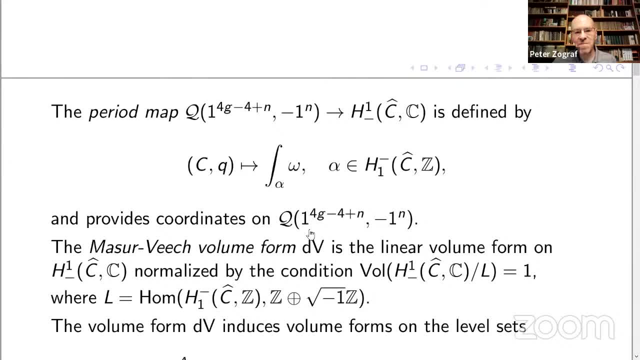 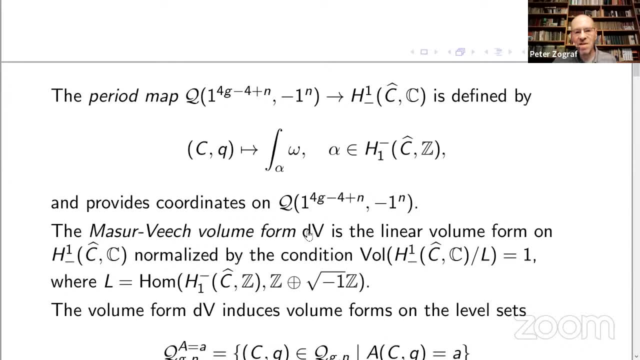 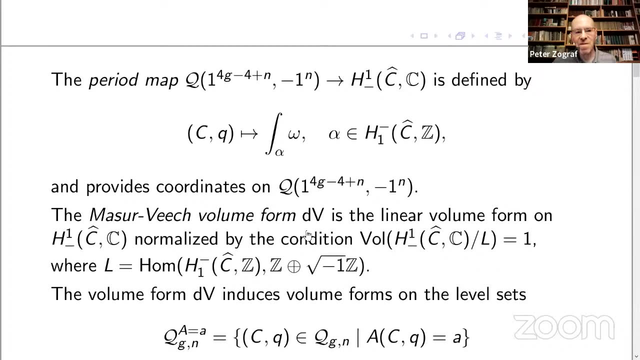 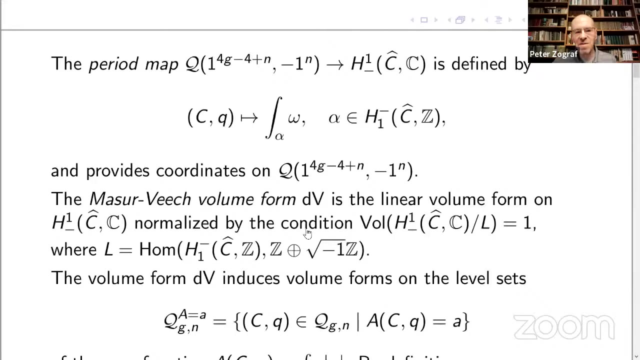 on the modular space of quadratic differentials. The measure of each volume form dV is the linear volume for H one minus on the homology group, H one minus of the odd cohomology or subspace in the cohomology with complex coefficients of C hat. 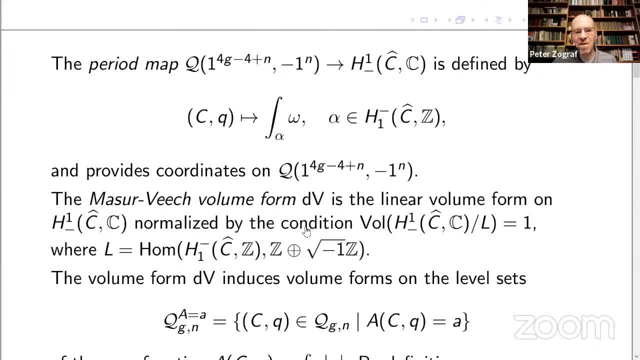 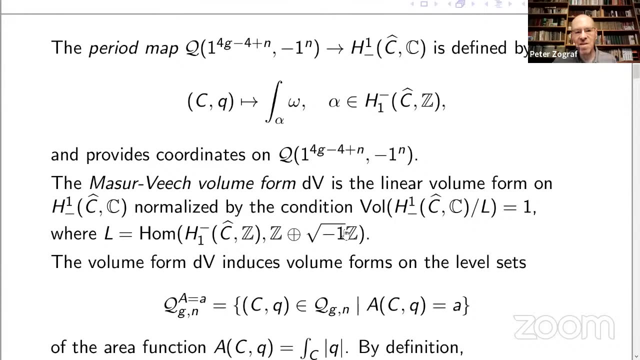 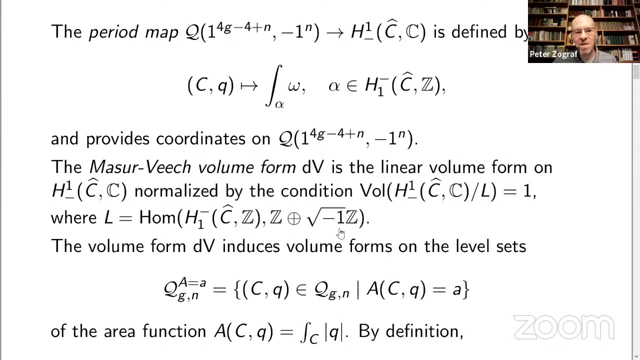 And it is normalized by the condition that the volume of the torus H one minus over L is one where L is a lattice of the torus, of the torus of the lattice of the linear maps, from H one minus to the group of Gaussian integers. 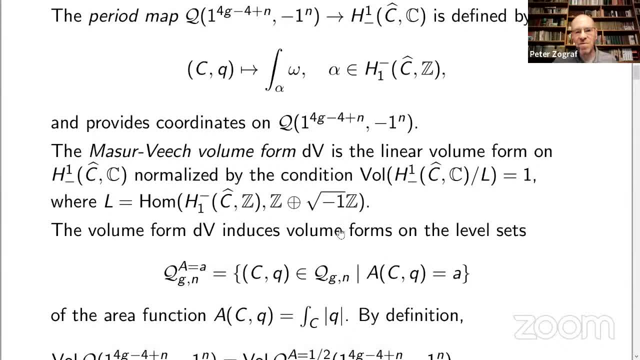 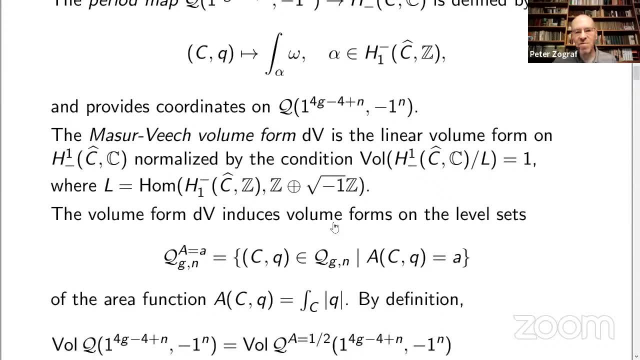 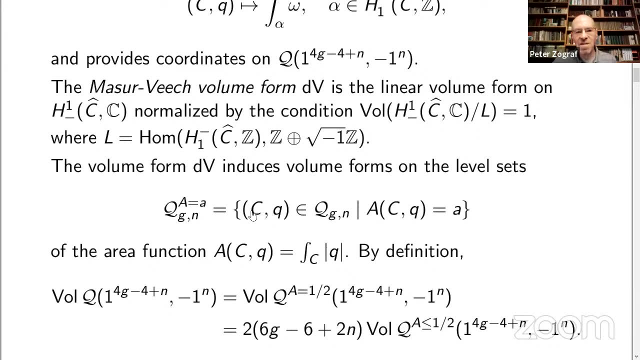 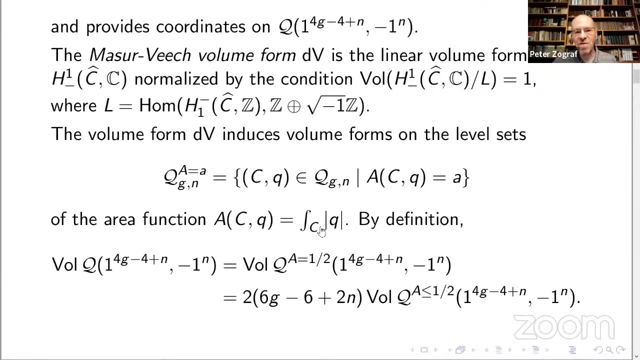 The volume form induces a volume force on the level sets Q, g, n at level A. that is the volume form of the H. one minus C hat plus H. one minus C hat minus L minus C hat minus L minus ot H. one minus G minus L minus. 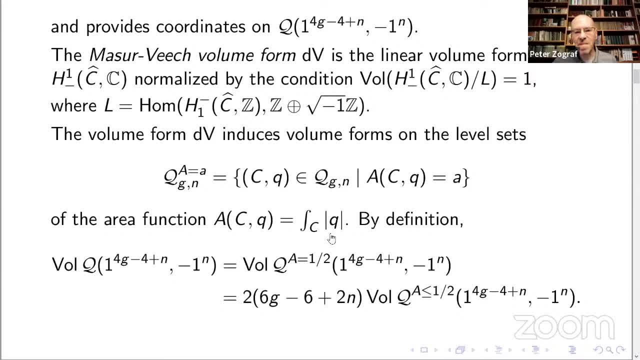 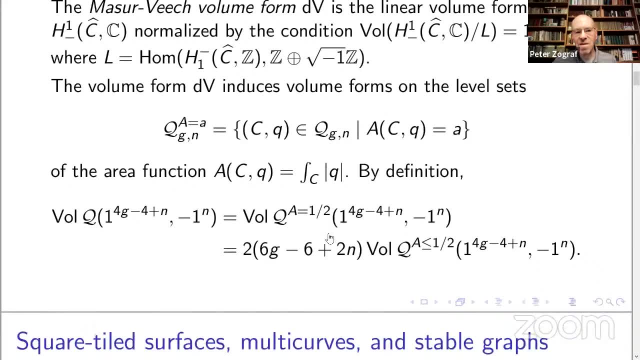 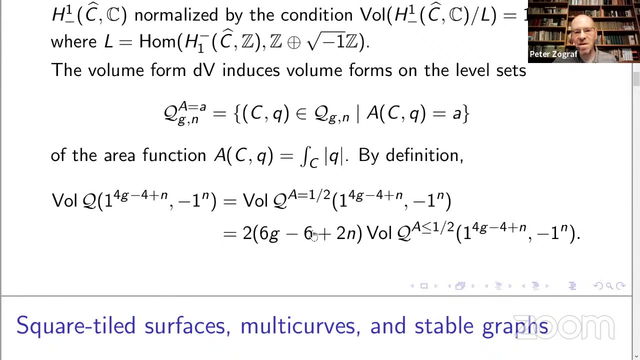 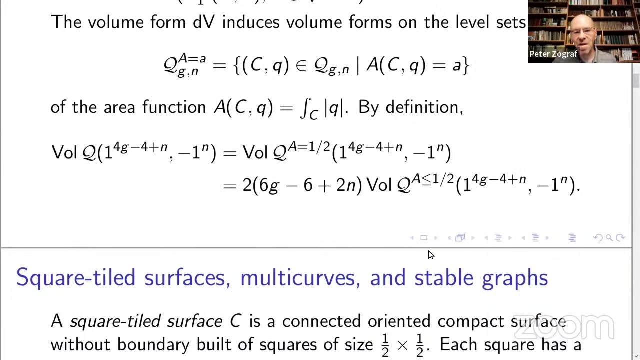 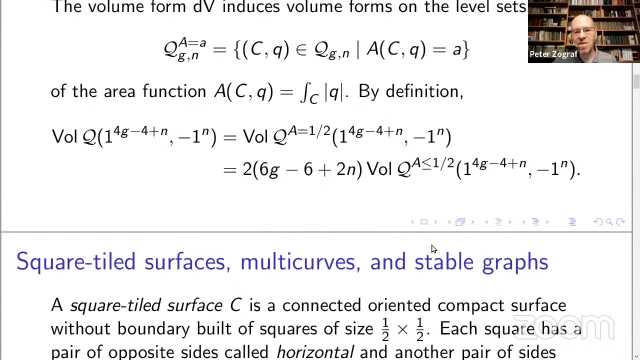 O points at the zeros, at the poles of Q. By definition, the volume of the principal stratum is the volume of the level set with area one-half, or it is the same, the volume of the disk bundle defined like this. So now I would like to establish a relationship. 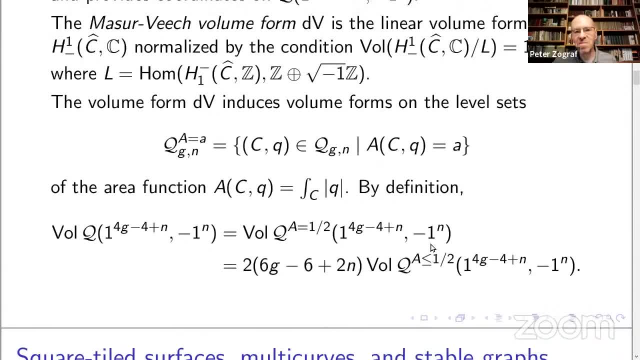 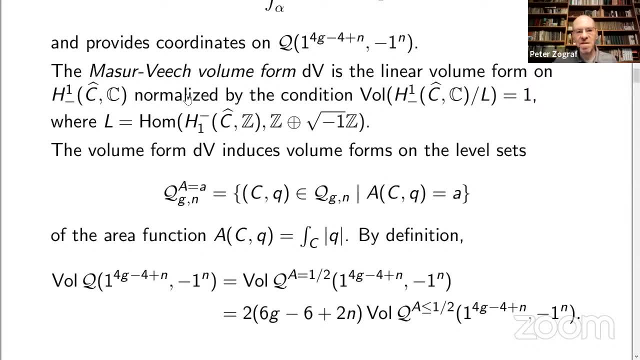 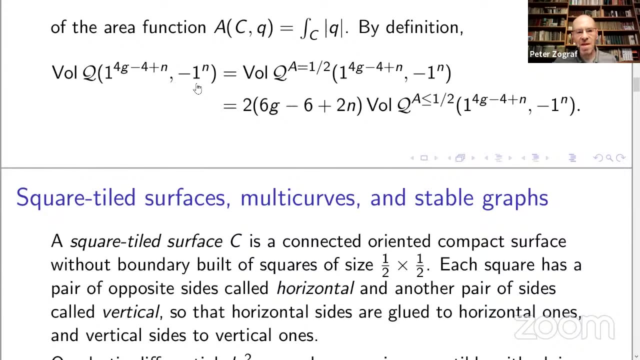 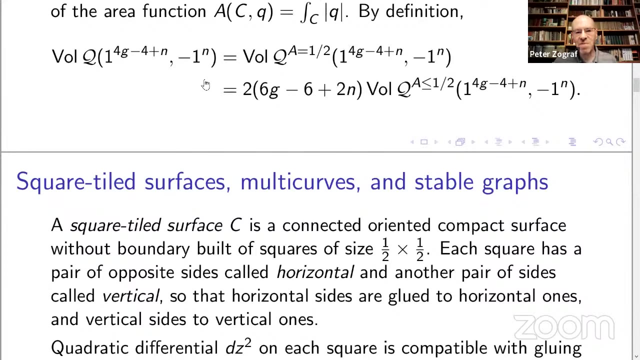 a correspondence between the lattice points- the points in the lattice L that was defined like this- and the so-called square-tile surfaces. The square-tile surface is a connected oriented compound surface without boundary, built of squares of size one-half by one-half. 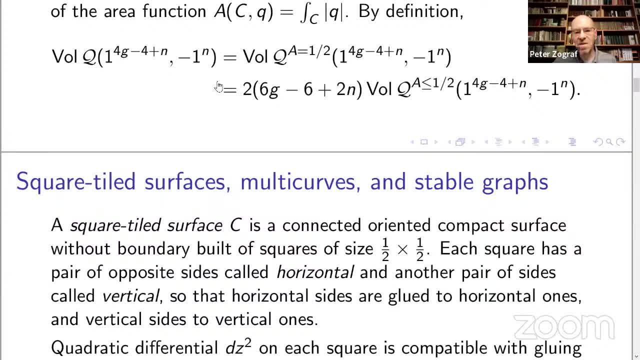 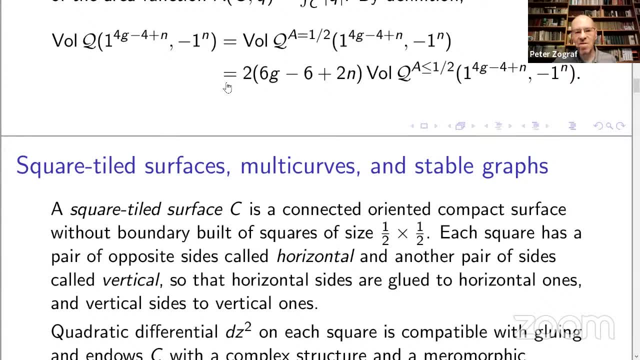 That's a quadrangulation of the surface with additional properties, that each square has a pair of opposite sides. One side is called horizontal and another pair of opposite sides is called vertical, So that the horizontal sides are glued to horizontal ones and vertical sides are glued. 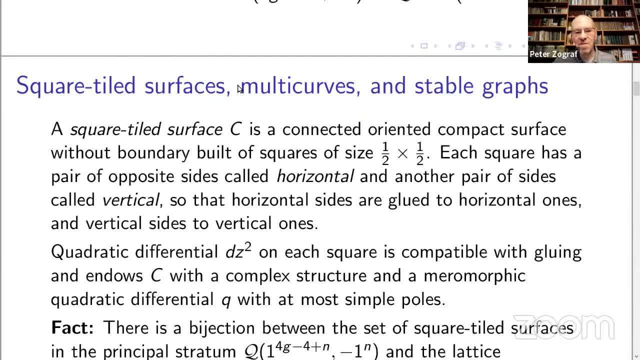 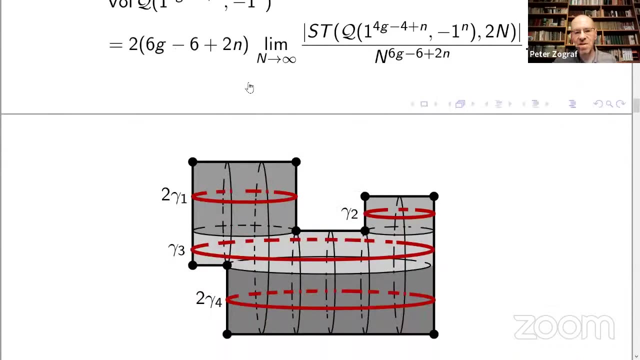 to vertical ones. A quadratic differential TZ, square on each square, is compatible with gluing and endos C with a complexity of one-half. So in this case we have a structure in the mirror-morphic quadratic differential Q with its most simple poles That can be seen on the picture here. This is a square-tile surface. 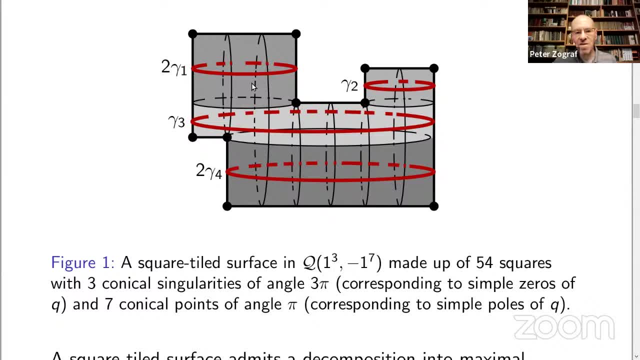 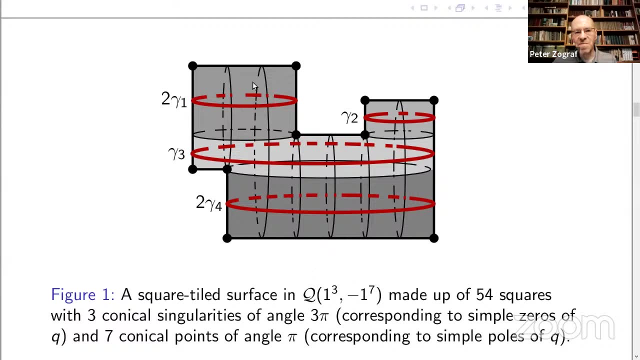 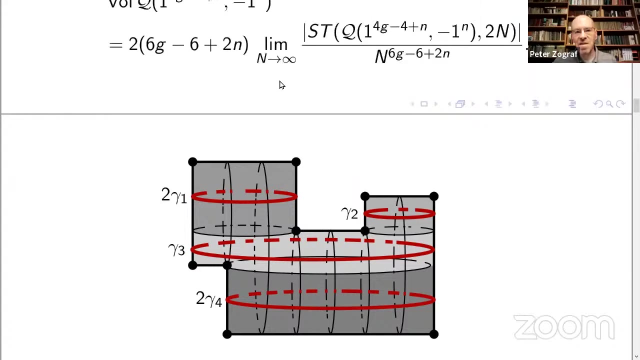 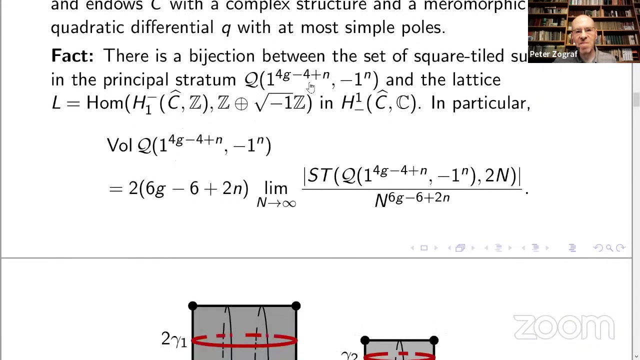 with three conical singularities of angle three, five that correspond to simple zeros of Q, and seven conical points of angle five corresponding to the poles of Q. So that's how a square-tile surface looks like, And an important fact is that there is a bijection between the set of square-tile surfaces in 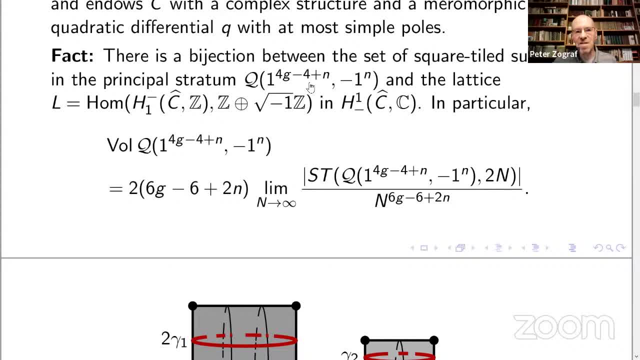 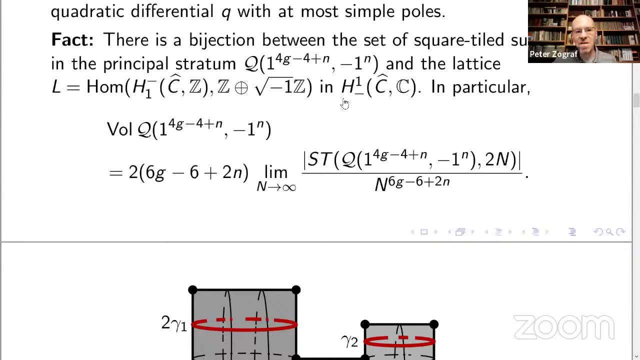 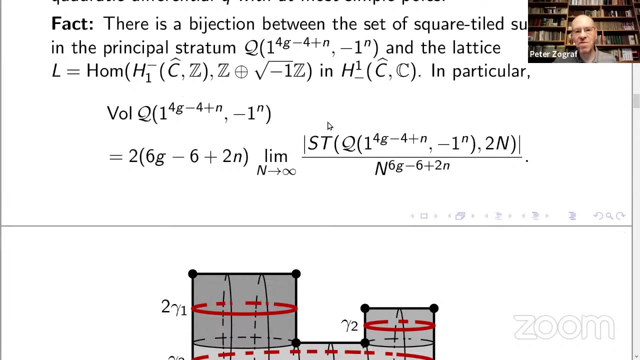 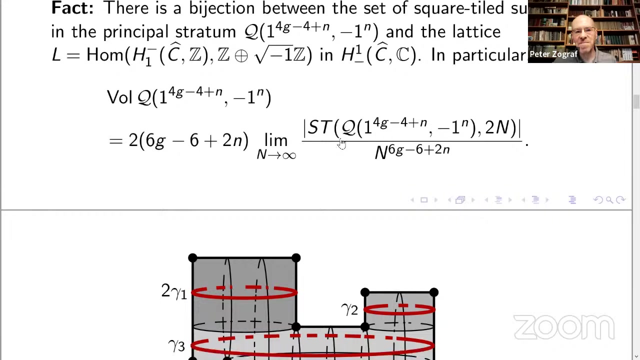 the principal stratum and the lattice L. in the first In particular, we can compute the volumes by counting square-tile surfaces in the principal stratum with at most two n-squares. The vertical bars mean the cardinality of this set and 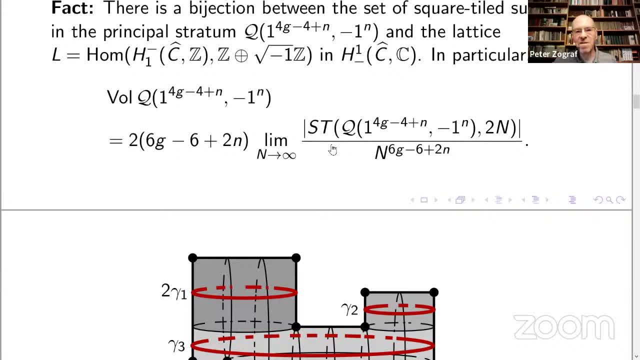 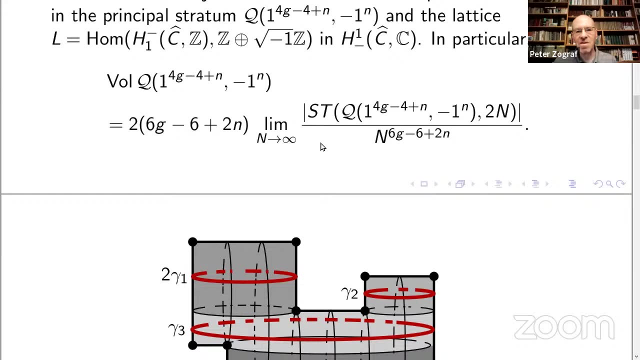 the limit of the set of square-tile surfaces in the set of square-tile surfaces is the constant size of the principal stratum. Also, the Rif enviesen tona of per chores used in the set of square-tile surfaces is the equivalent of the full requests and combinations. 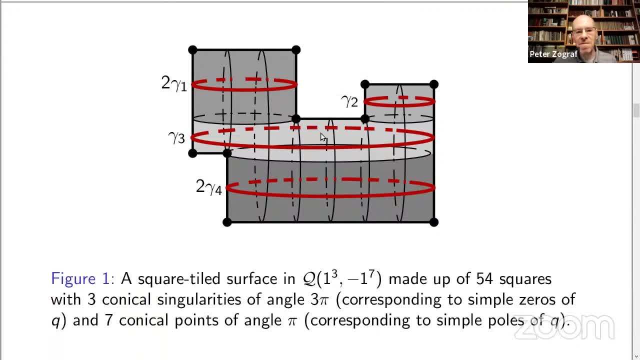 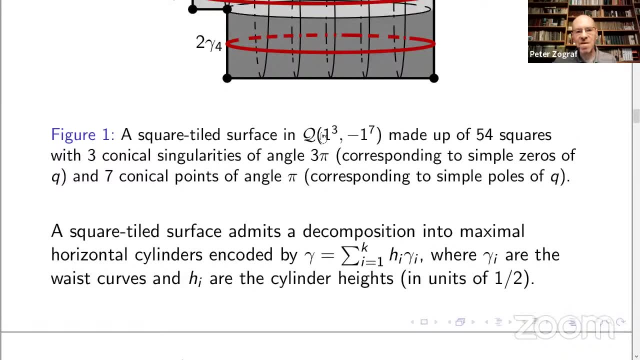 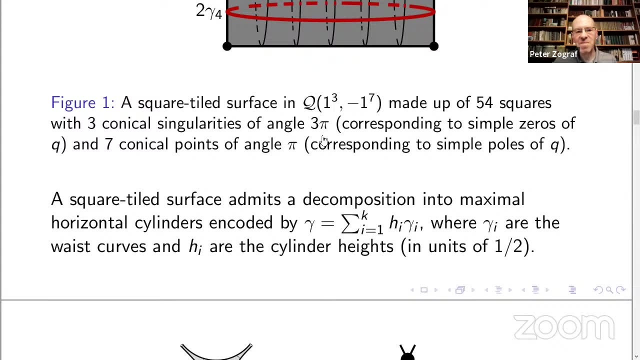 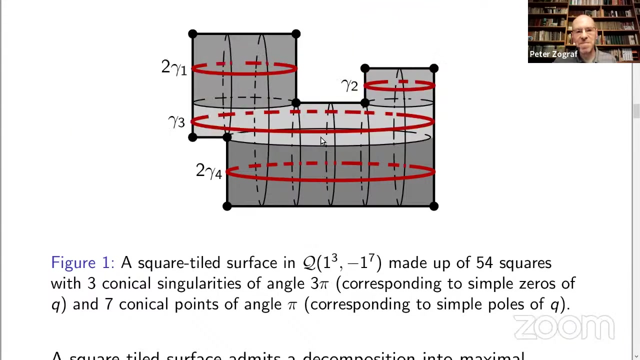 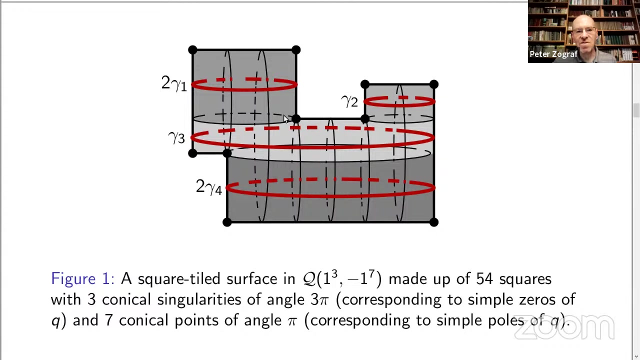 And this constant volume is an equivalent to the interval state of Castings mínimum n, n minus x square tile surfaces- is that it admits a decomposition into maximal horizontal cylinders included by the waist curves of the cylinders and their heights. So on this picture, the first cylinder has circumference 6 and height 2.. 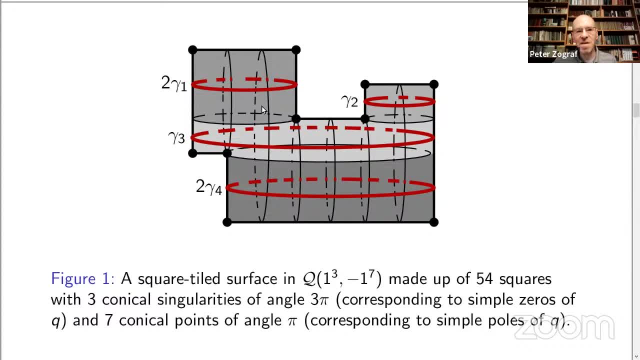 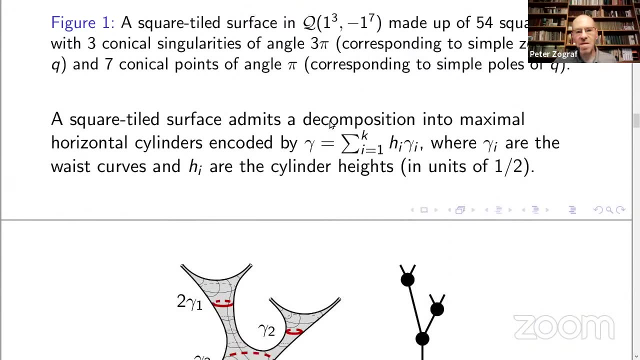 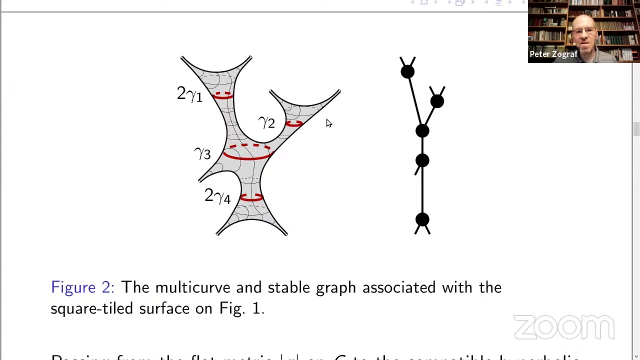 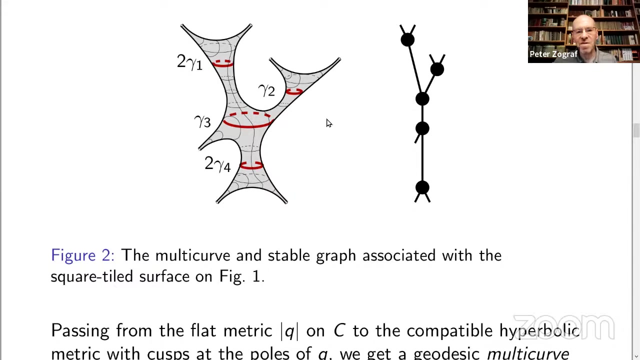 It is encoded by the symbol 2, gamma 1.. The second cylinder has circumference 4 and height 1, and so on. Now there is another object related to square tile surfaces, That's what is called a geodesic multi-curve. 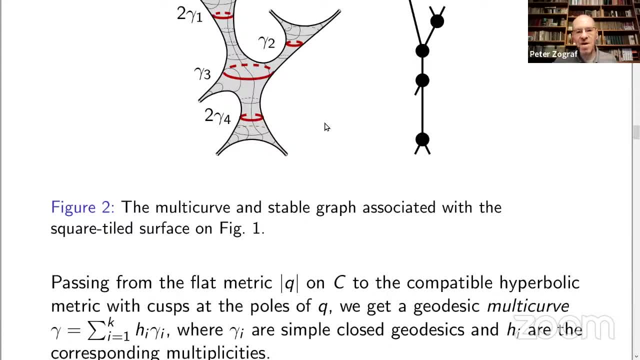 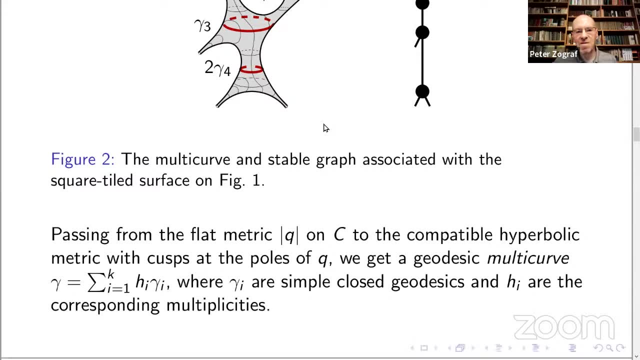 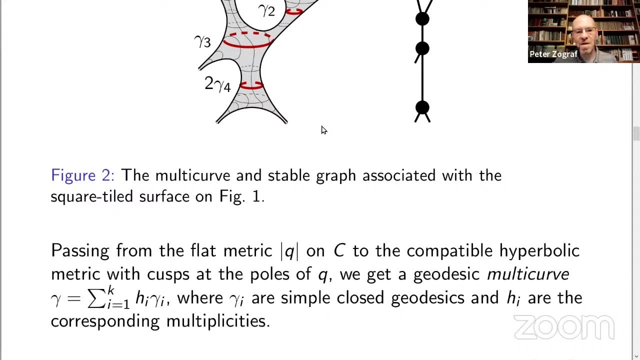 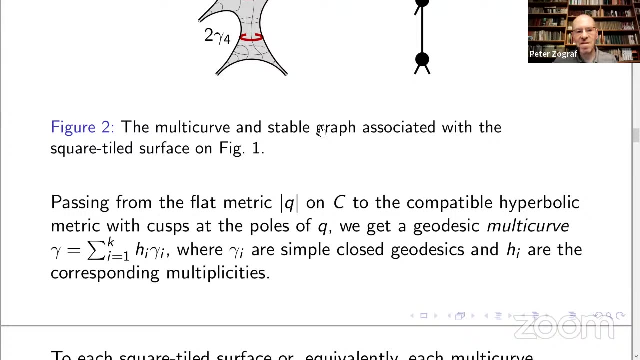 We can end of C with the compatible hyperbolic metric with cusps at the poles of Q And the waist curves of cylinders form a geodesic multi-curve gamma written as: the sum of gamma sub i, h, i sum of i from 1 to k, where gamma i are simple closed geodesics. 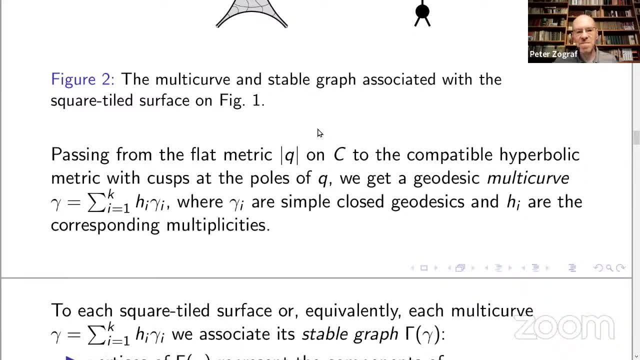 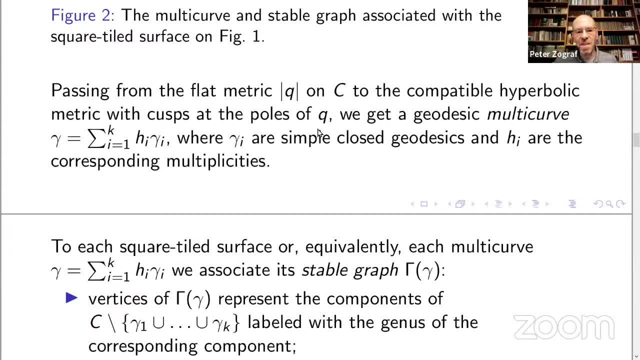 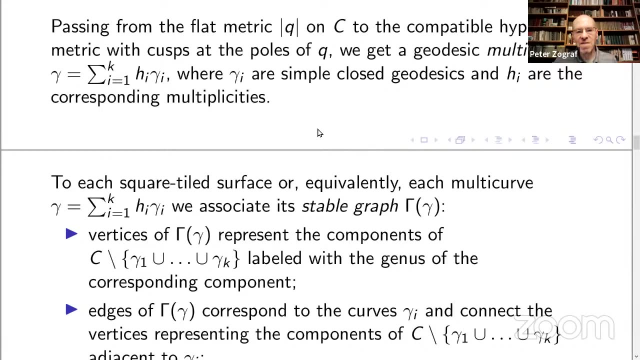 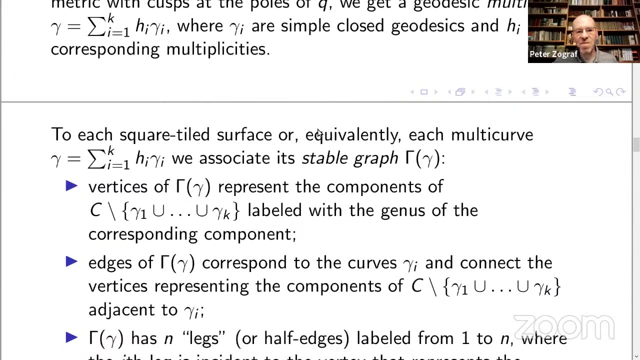 and h i are the corresponding multiplicities To each square tile surface or equivalent to each multi-curve. we associate its stable graph: gamma, big O, gamma. The stable graph is the collection of the following data: The vertices of it represent the components of the complement of the union of the irreducible. 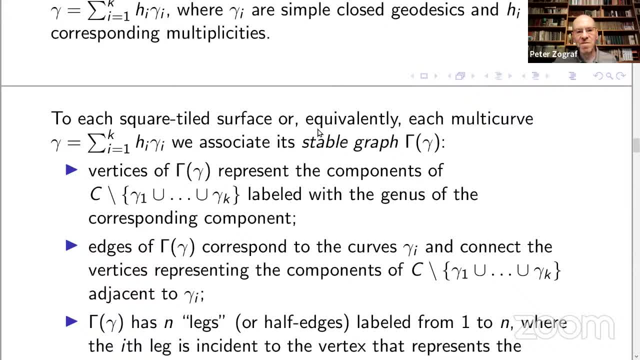 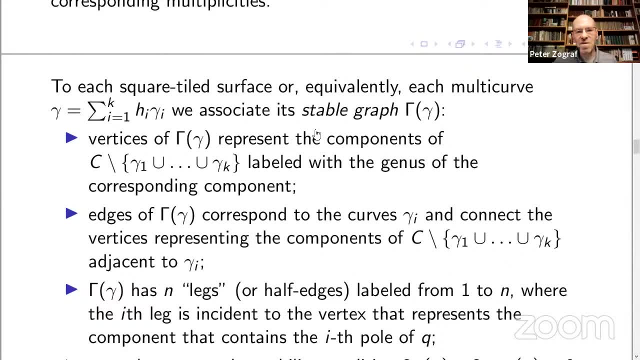 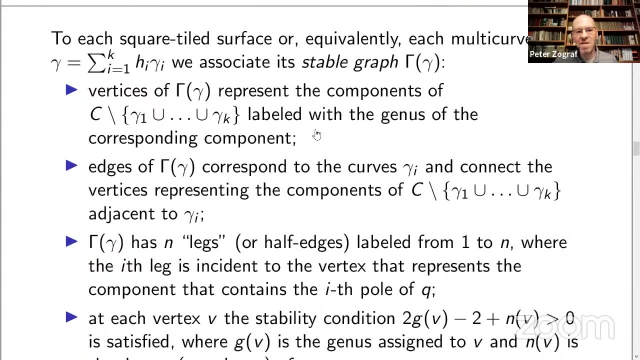 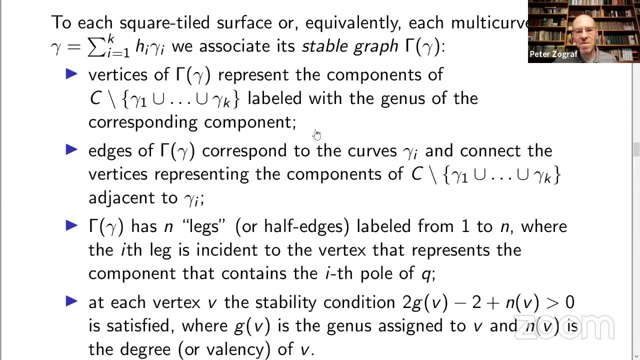 components of the multi-curve. Thank you. The edges of gamma correspond to the curves to the irreducible components of the multi-curve and connect the vertices representing the components of the complement to the union of irreducible components of the multi-curve. 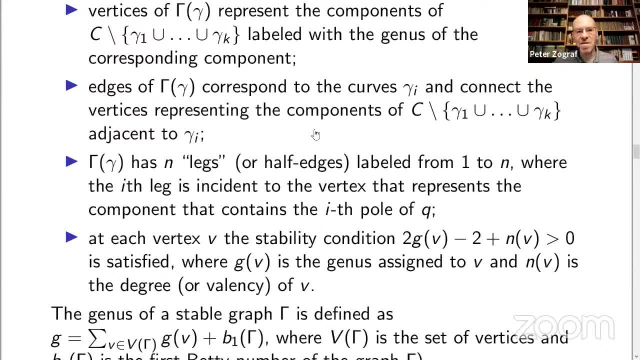 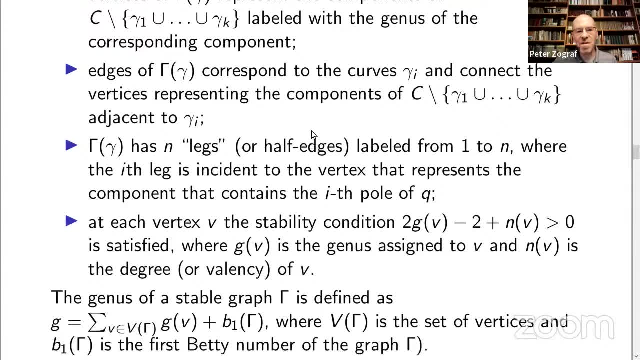 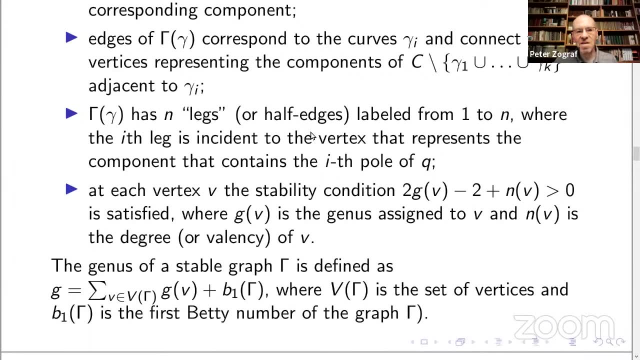 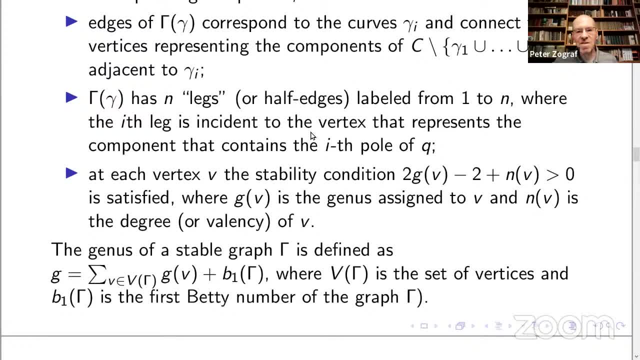 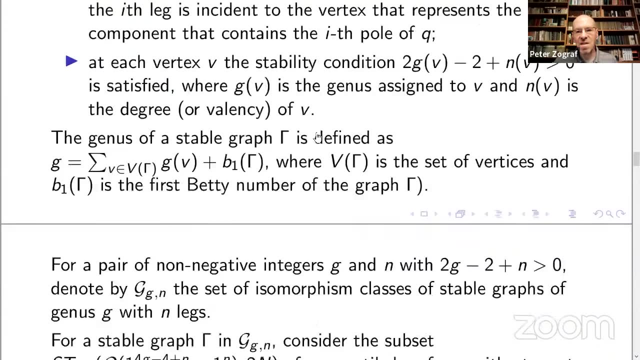 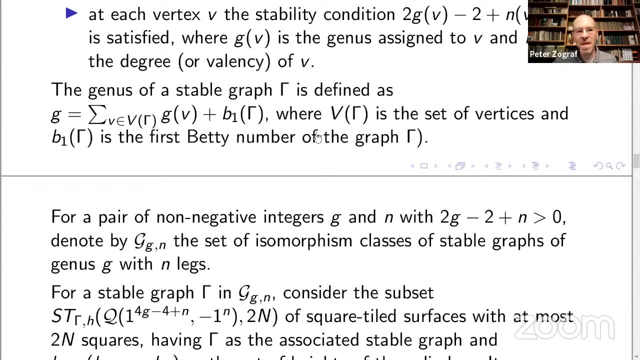 And at last, at each vertex, the stability condition is satisfied, where gamma – oh sorry, where g of v is the genus assigned to v and n of v is the degree of valency of the vertex v, The genus of the stable graph gamma. 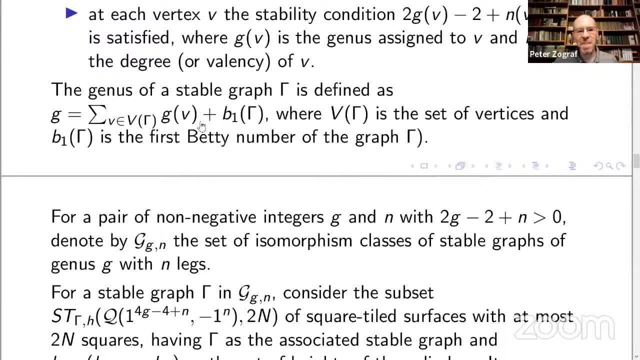 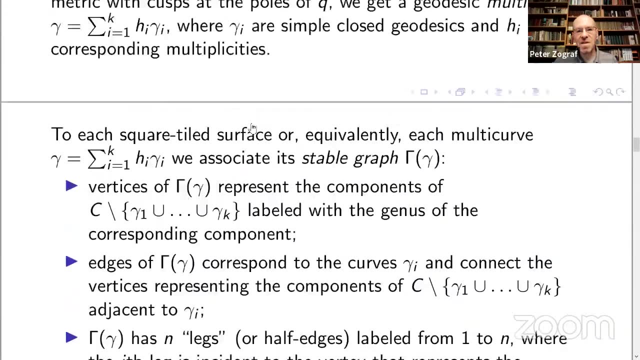 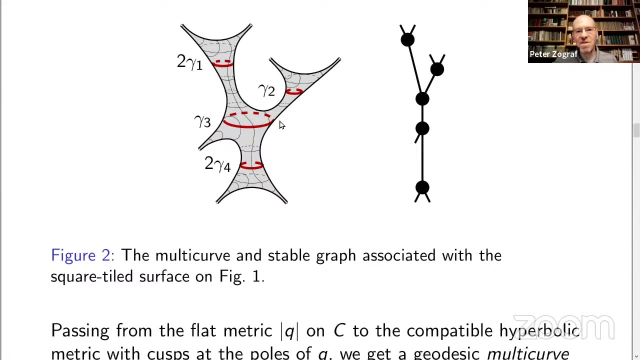 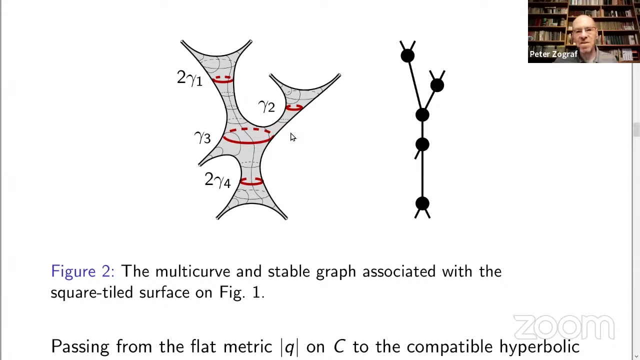 is defined by this formula, where v of g is the set of vertices of gamma and v1 of g is the first 30-number of the graph gamma. So on this picture, all the multi-curve and the corresponding stable graph. 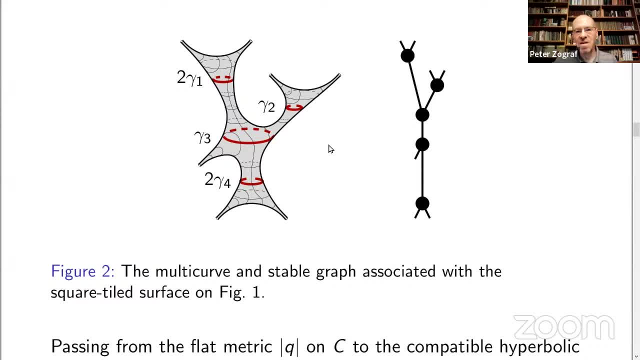 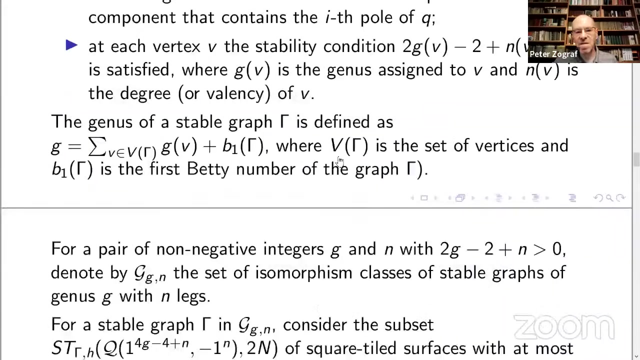 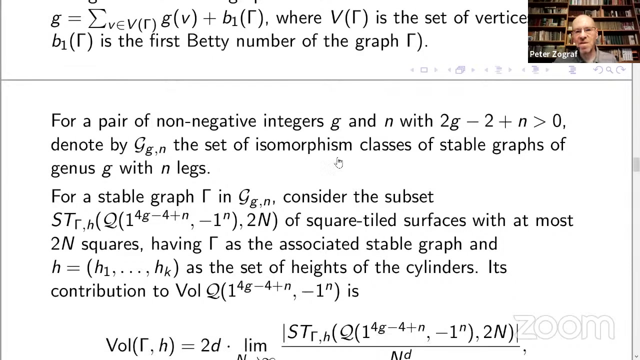 all labels are at 30 cycles. In the integral to 1, there are 4 edges and 7 legs For a pair of non-negative integers, g and n. we'd be conditioned that 2g minus two plus n is one. 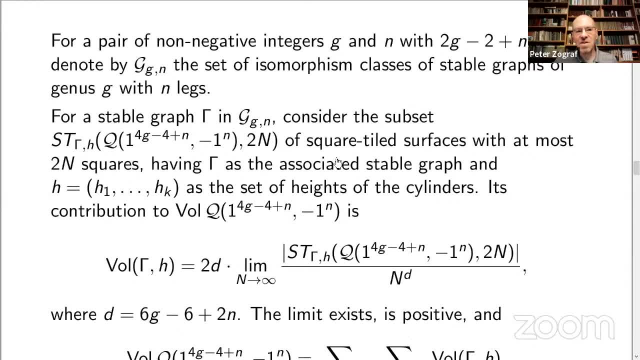 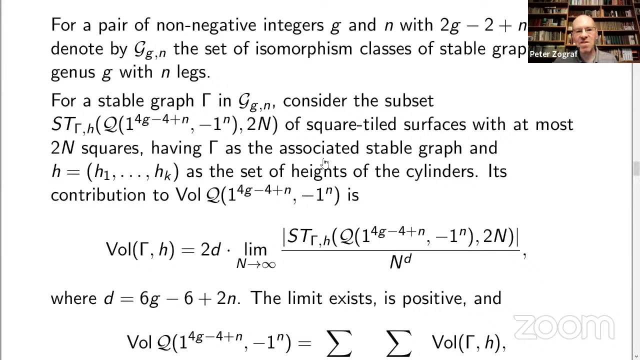 larger than zero. denote by g- gn the set of isomorphism classes of stable graphs of genus g with n legs. For a stable graph, gamma in g? gn, consider the subset of square tile surfaces with at most two n squares having gamma as the associated stable graph and h as the 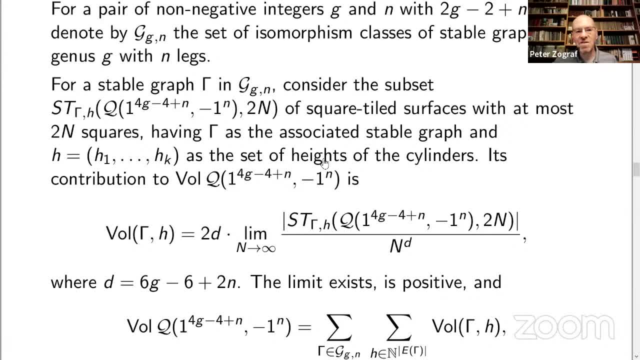 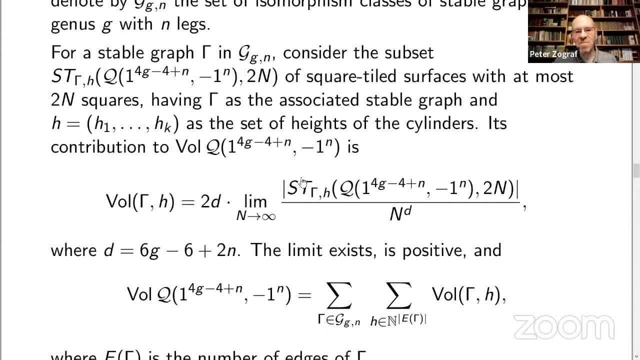 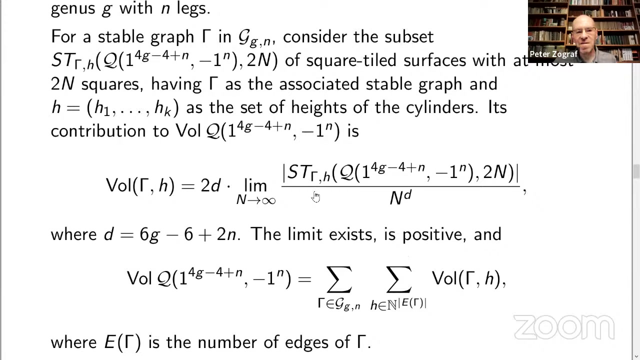 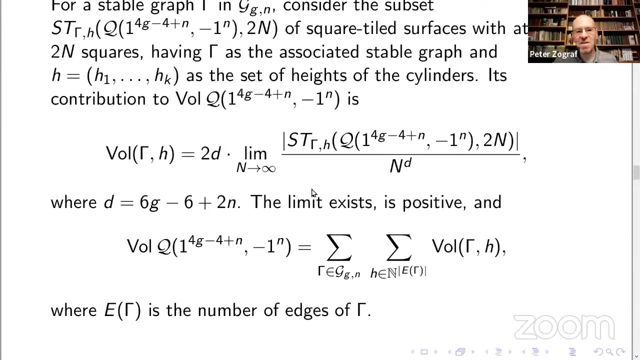 set of highs of the cylinders. This contribution to the volume of the principle stratum is given by the limit, when n tends to infinity, of the number of square tiles. Here d is equal to 6g minus 6 plus 2n is the dimension of the modular space and the 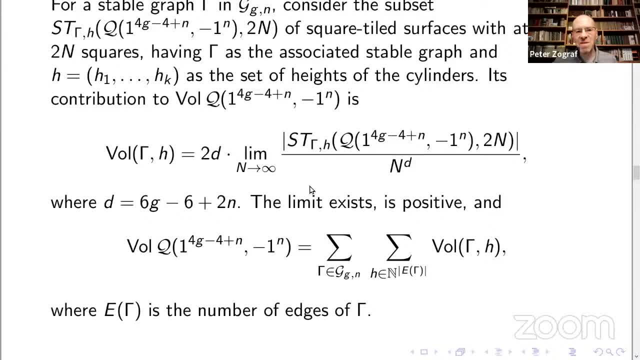 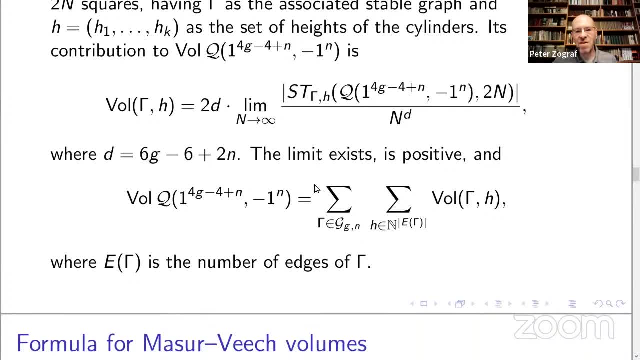 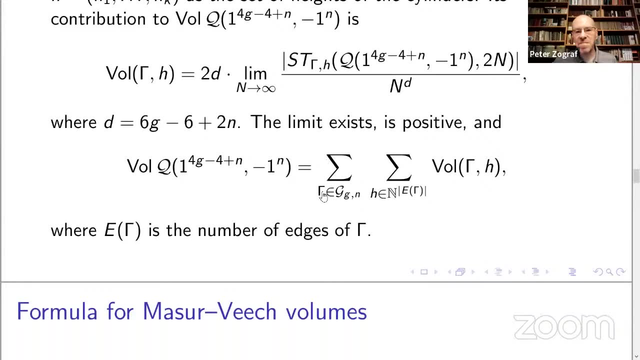 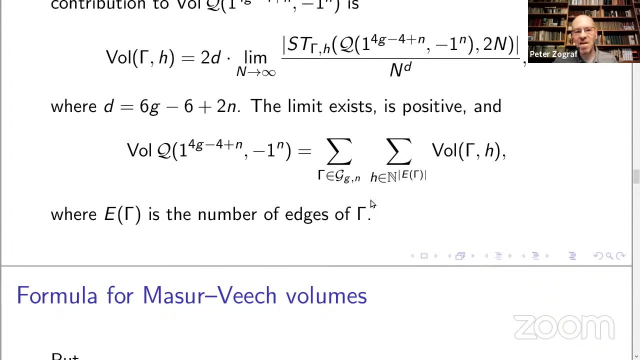 dimension of quadratic differentials. This limit exists, is positive and the volume can be written under the sum over all stable graphs, the sum of the set of highs, of the volume contributions of each stable graph. Here e of g is the number of edges of gamma. 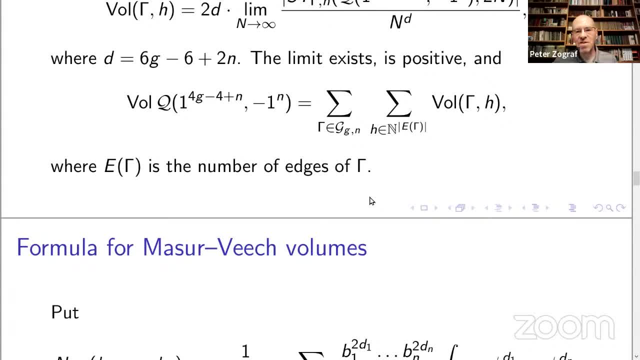 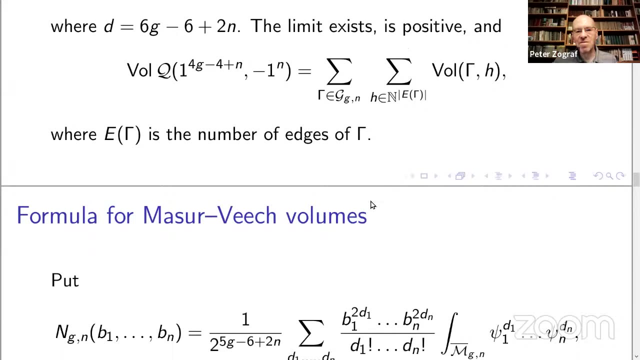 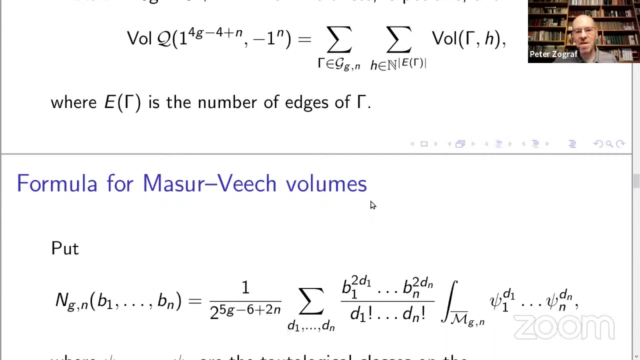 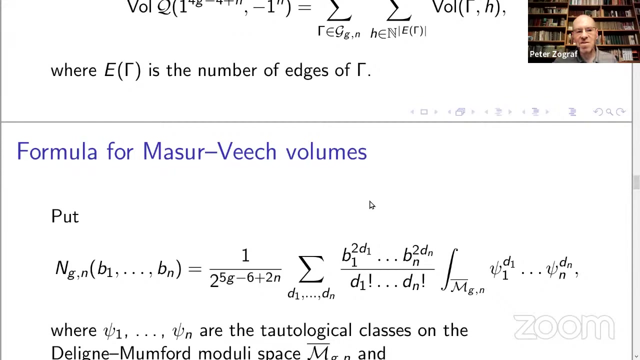 Now the first application of this correspondence between lattice points, square tile surfaces, geodesic multicurves and stable graphs allows us to deduce a formula for major reach volumes of the modular spaces. For that we need to introduce certain polynomials- mg- of variables v1 to vn that are given by: 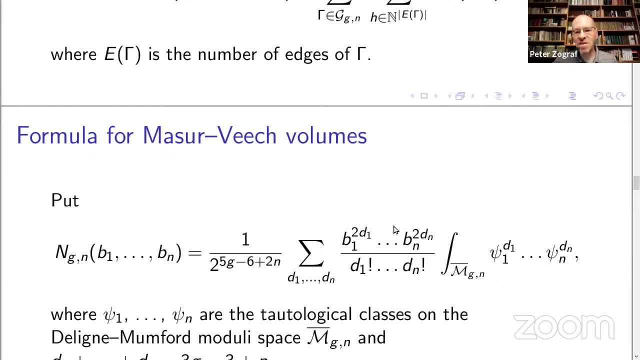 this formula: Here the integral over the Dillin-Marford modular space- mg of the psi classes, And here the integral over the Dillin-Marford modular space- mg of the psi classes. And here the integral over the Dillin-Marford modular space- mg of the psi classes. 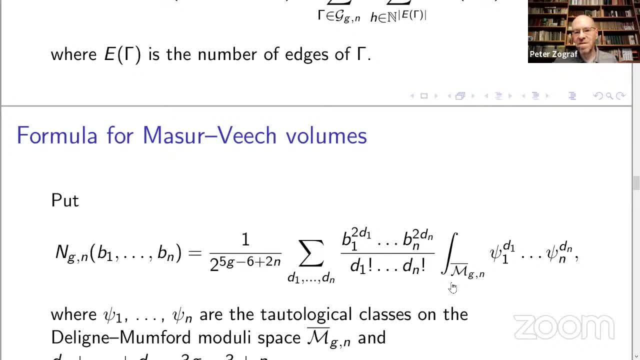 Here the integral over the Dillin-Marford modular space, mg of the psi classes And the interval over the Dillin-Marford modular space mg of sin瓜 s mg of an integral over�, and these designed numbers are of payment for the. 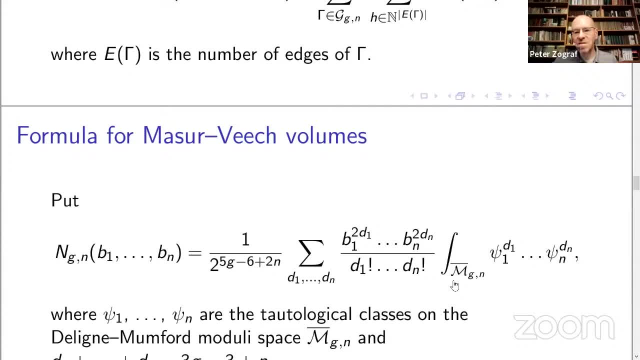 española robots' PCSR Users. so to chess. And this formula is using here these international variables to王 ile In the pyramid of digestible matter of space, these Storage-band additions are rise an, despite the hierarchy of Korteweg-De Vries equations. 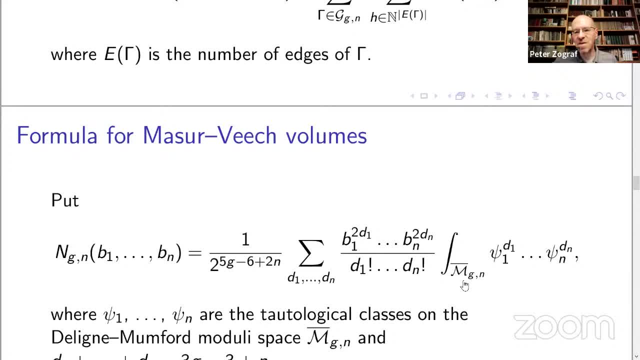 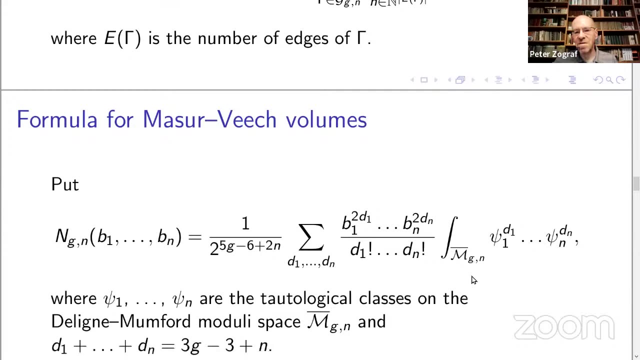 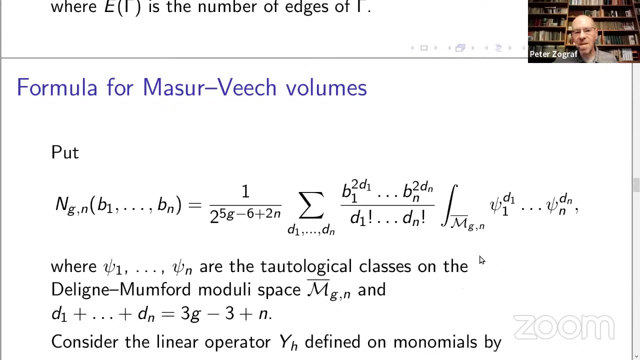 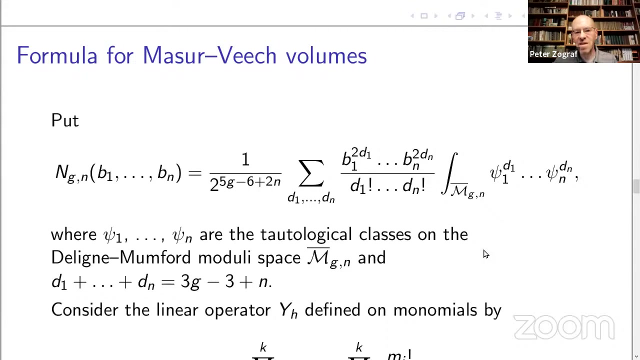 This conjecture was proven by Kancevich and then by many other people. And these numbers, they are relatively well studied and they appear as a top degree coefficient in the latest point count polynomial of Paul Norbury. So yes, Psi one to Psi n are the tautological classes. 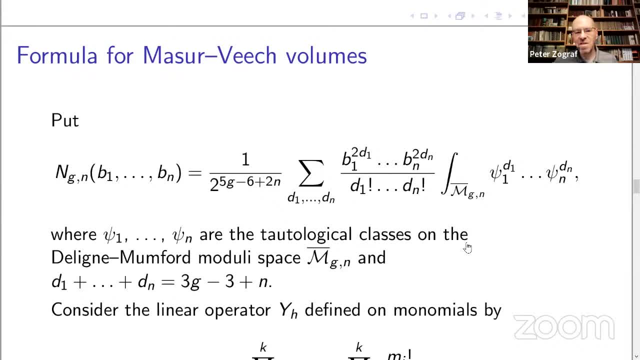 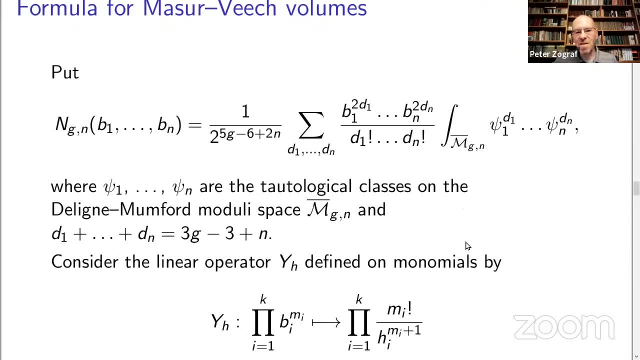 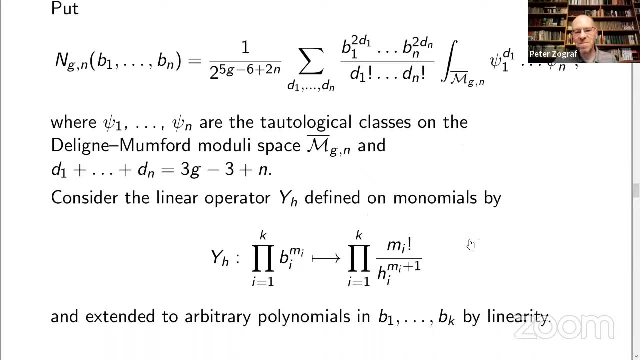 on the dealing map of multiple space, And the sum of these should be equal to the dimensions of the Korteweg-De Vries equations. And this is a very good representation of MGM. Now consider the linear operator YH, defined on monomials by this formula: 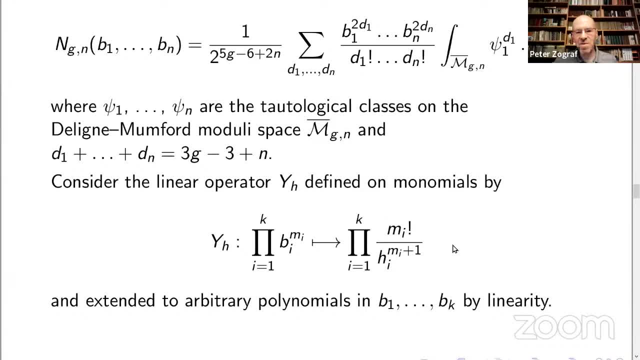 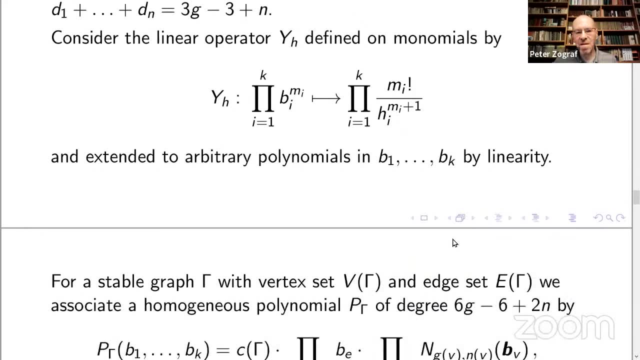 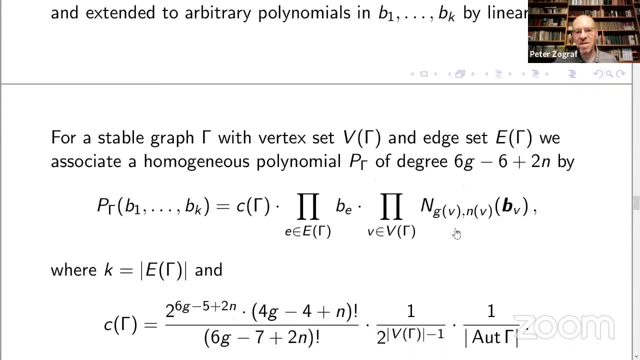 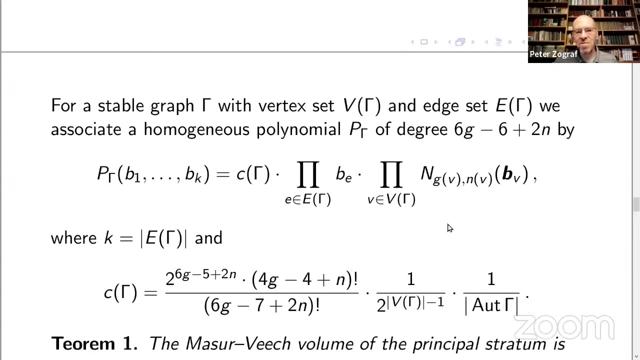 and extended to arbitrary polynomials V1 to VK by linearity For a stable graph gamma with vertex set V of gamma gamma and the edge set E of gamma associate a homogeneous polynomial P gamma of degree 6G minus 6 plus 2 by the formula: 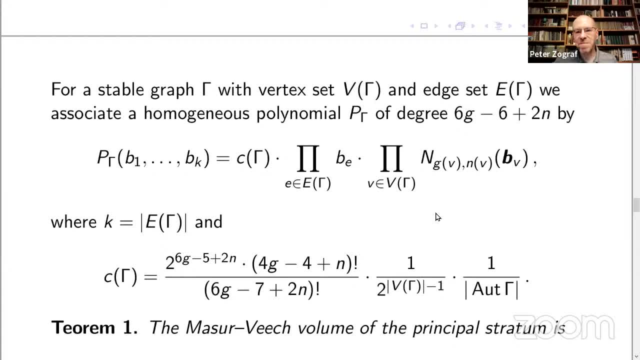 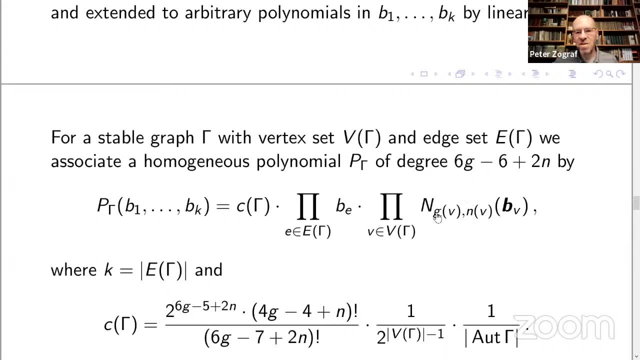 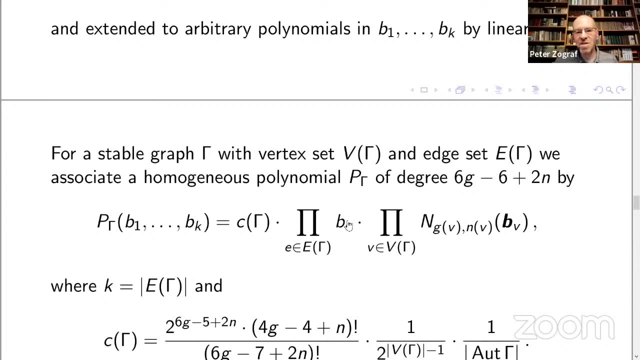 By this formula it's up to a certain coefficient given by the product over all edges. To each edge we assign a variable B E times the product over all vertices and to each vertex we assign the polynomial N, G, N. It was just defined where B bold. 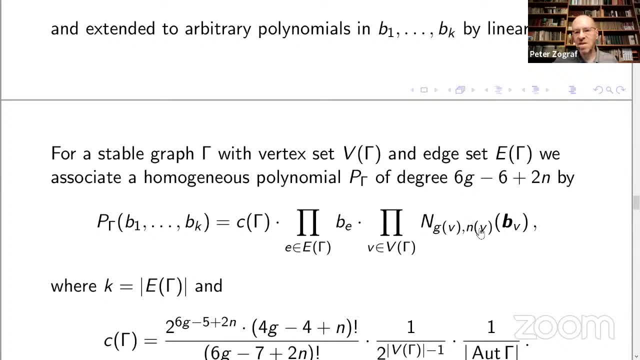 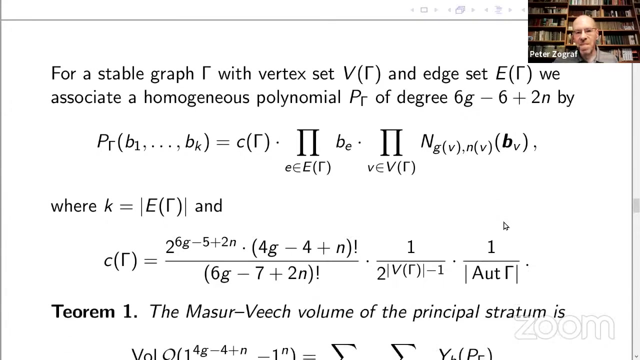 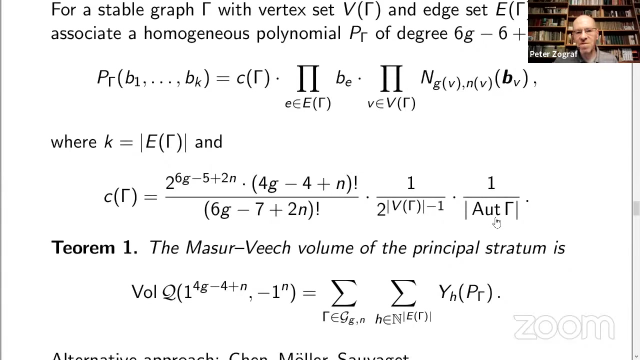 denotes the set of variables- N, G, N- designed to half edges. We assign a variable to half edge of a full edge and we assign 0 to a leg. So, in terms of this polynomial, to measure which volume of the principal stratum is given by the formula: 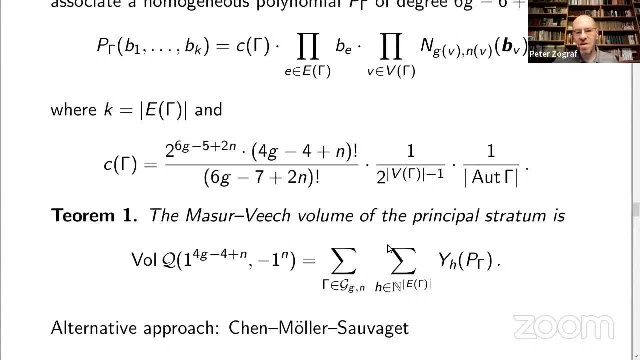 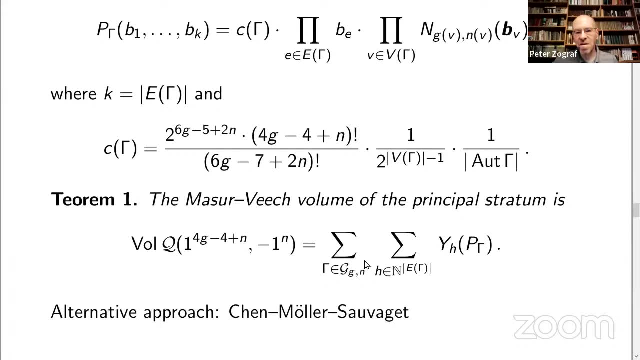 So we could give the new the sum over whole set of graphs of genus G with N legs, of genus G with N legs, also N edges, also N edges, of only N edges, of only N edges. So yet so and so. 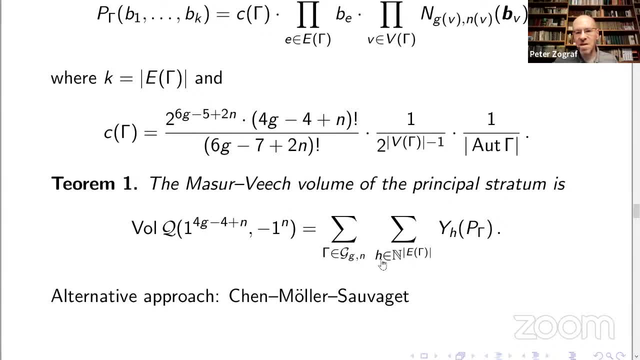 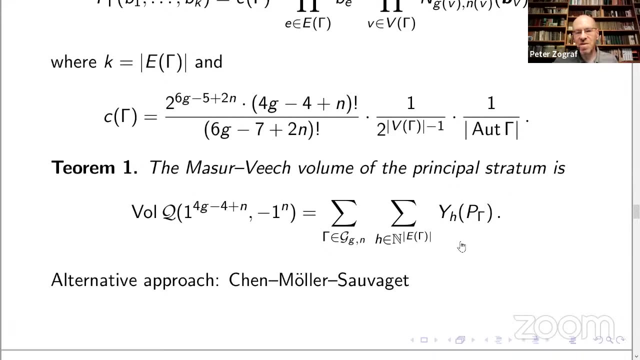 You know all the sum of actual numbers as the sum of all the data provisions in our fieldtaking, sum over all sets of highs of the operator yh, applied to the polynomial p gamma. So this formula has some advantages, Namely it gives the volume: 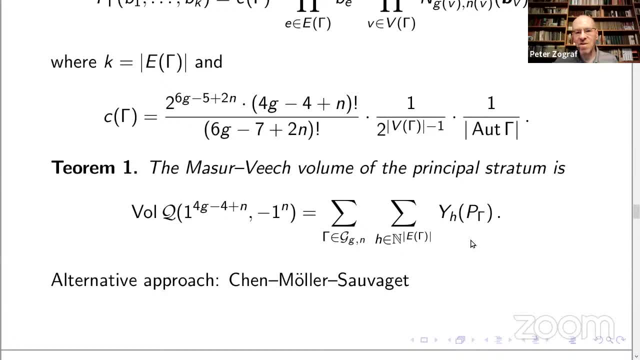 as the sum of individual contributions over stable graphs. But on the other hand, the number of stable graphs grows rapidly with g and b, and it's not very well suited for computing these volumes. There is an alternative approach to the volumes of modular space of quadratic differentials. 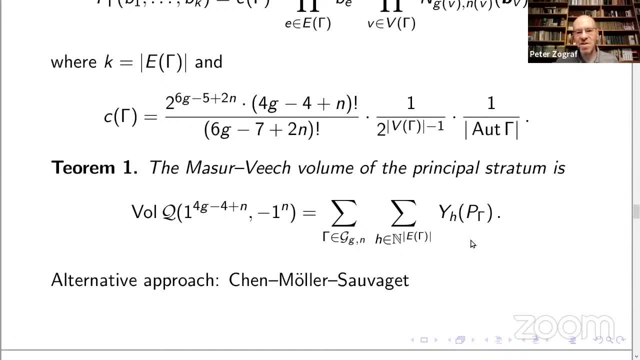 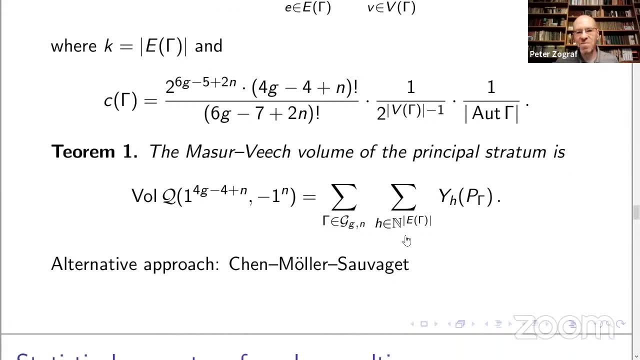 That is due to Chen, Noeller and Solange. They derived a quite different formula for these volumes using intersectional theory on the modular space of quadratic differentials, And they expressed these volumes in terms of the so-called linear Hodge integrals. 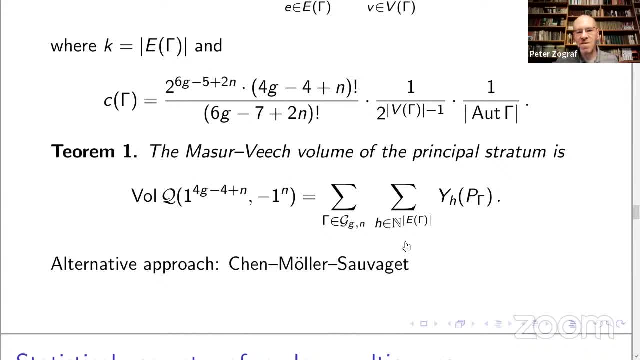 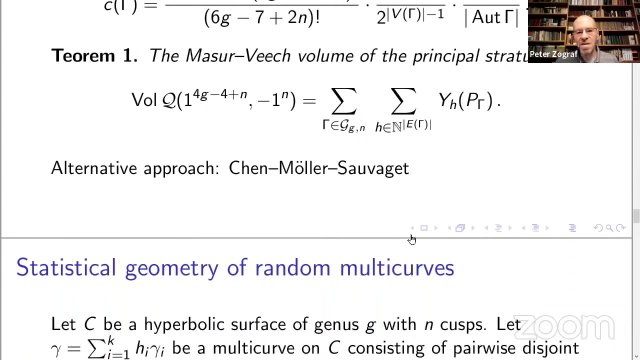 over the modular space of quadratic differentials. What is interesting is that both formulas give the same values for the volumes, but at least I don't know of any direct proof that these two formulas give the same things. Thank you. Now another application is to the statistical geometry of random multicolors. 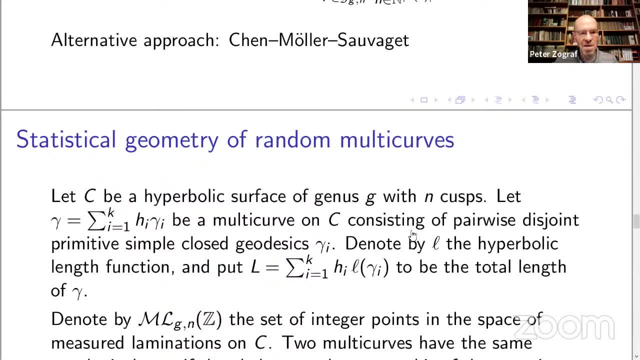 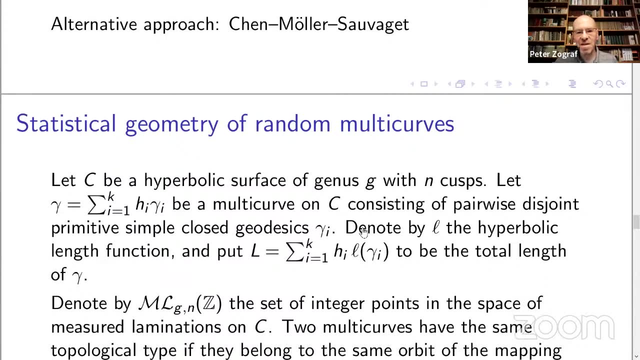 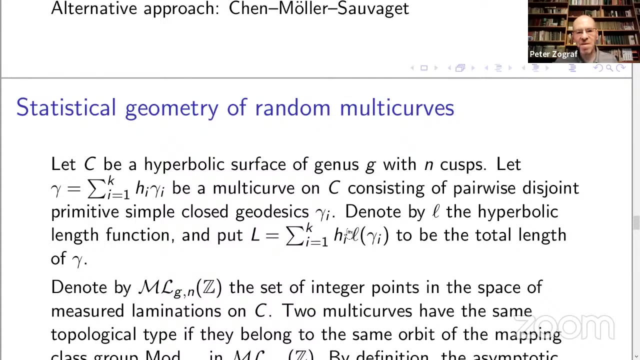 So let C be a hyperbolic surface of genus G with n cusps, And let gamma be a multicolor C consisting of pairwise disjoint, primitive, simple, closed geodesic gamma. I. Now denote by L the hyperbolic length function and put L big, equal the sum over irreducible components. gamma I of lengthless multiplied by multiplicities. 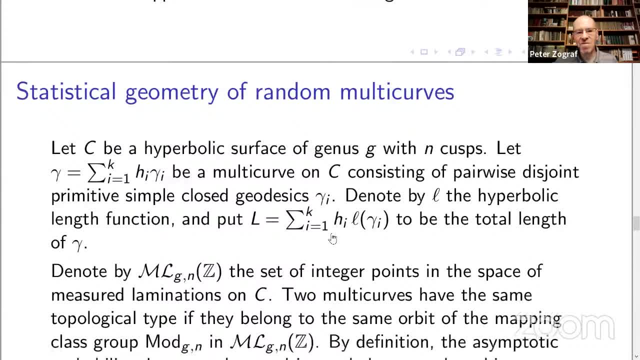 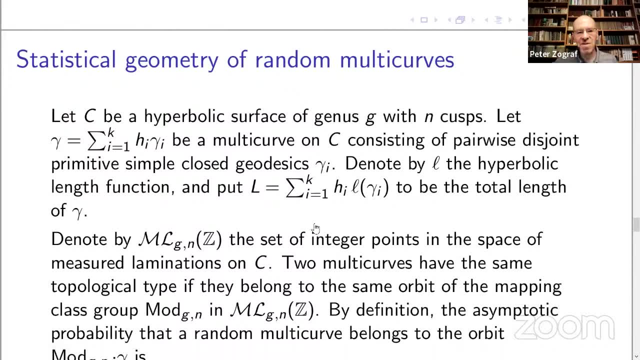 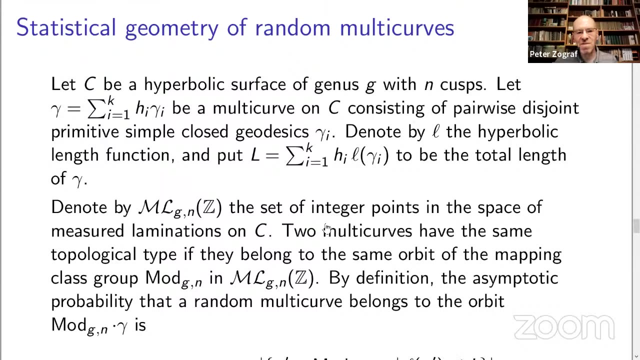 So this L is called the total length of the multicurve gamma Now denote by MLGN of Z. So this is the set of integer points in the space of measured laminations On C. two multicurves have the same topological type if they belong to the same orbit of the methane class group. in the space of integer points, 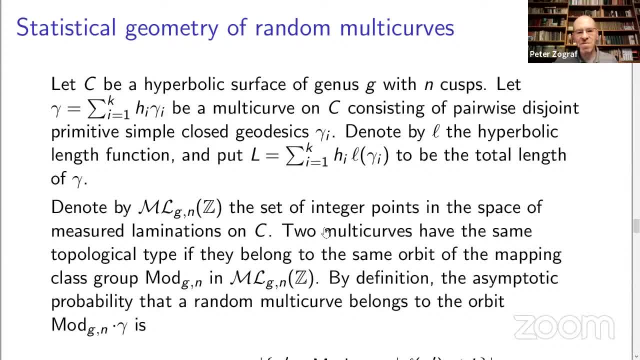 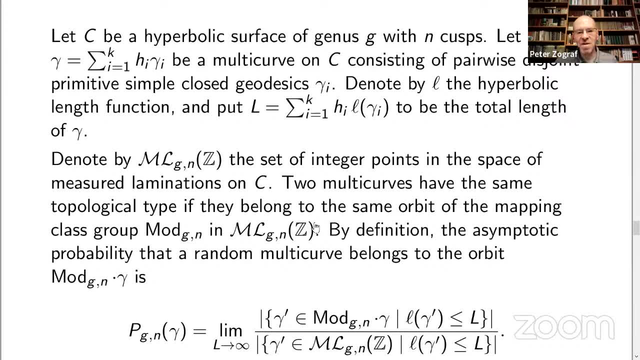 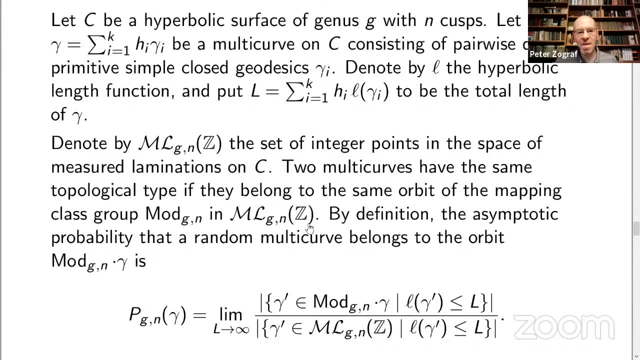 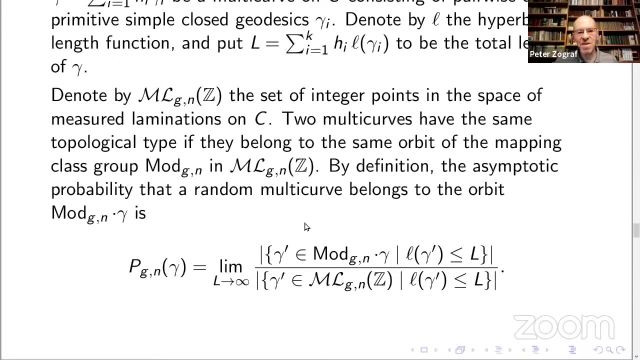 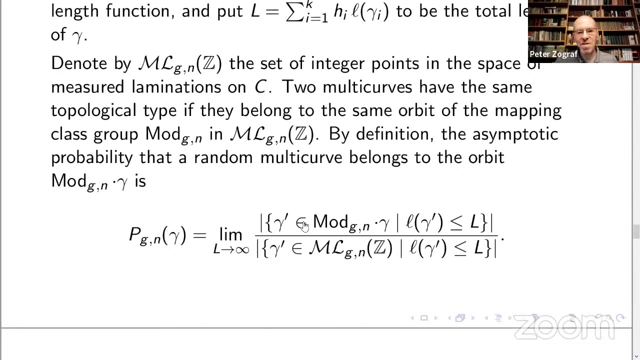 and on the set of integer points in the space of measured laminations. By definition, the asymptotic probability that the random multicurve belongs to the orbit of the modulo group. modul Gn is the limit of the ratio of the number of multicurves in the orbit of gamma that is not longer than L over the set of integer points. 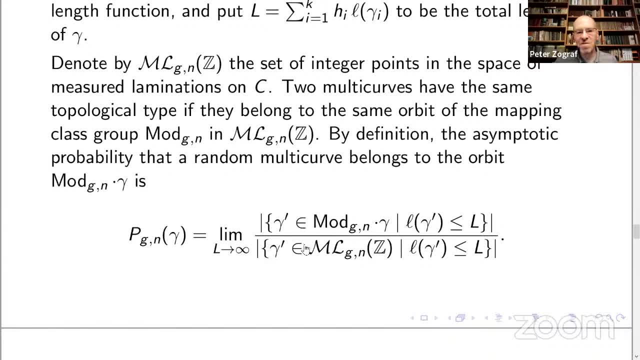 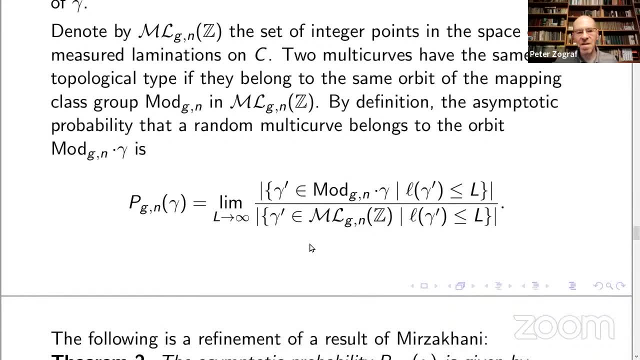 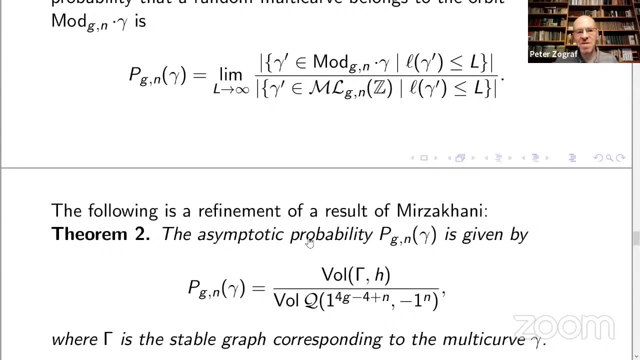 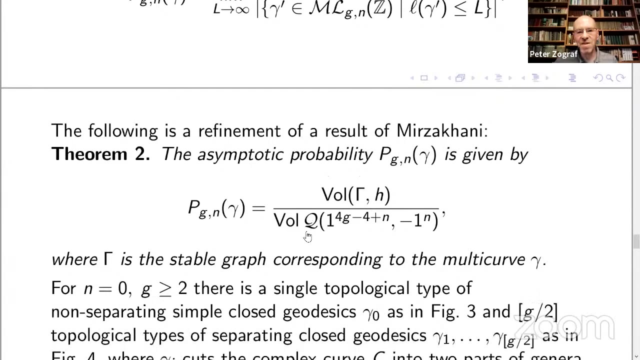 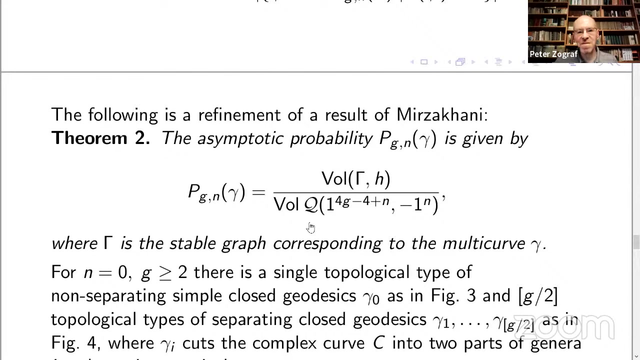 So the number of all multicurves whose length doesn't exceed L. The following formula is a refinement of a result of Mirza Hany and describes this probability in terms of the volume contribution of stable graphs, namely the asymptotic probability PGN of gamma is given by the ratio of the volume contribution from the stable draft. 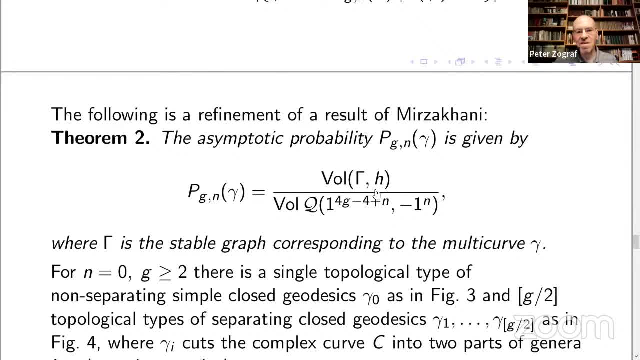 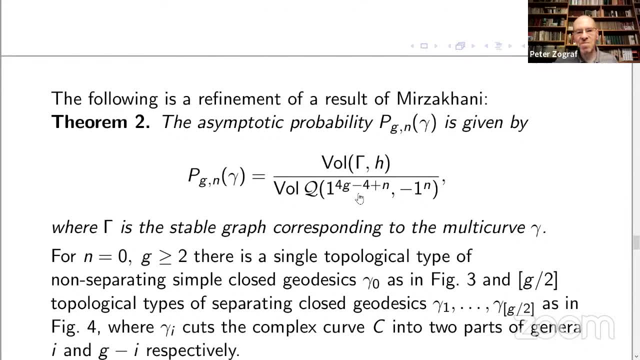 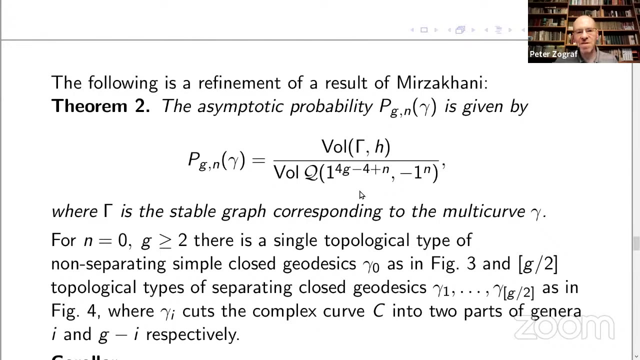 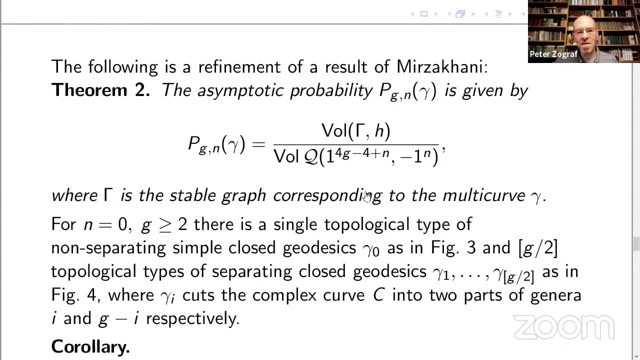 gamma with the set of height h over the volume of the total stratum of quadratic differential. Here, as I said, gamma is the stable graph corresponding to the multi-curve. gamma For n equal 0 and g is greater or equal to 2, there is a single topological type of non-separating. 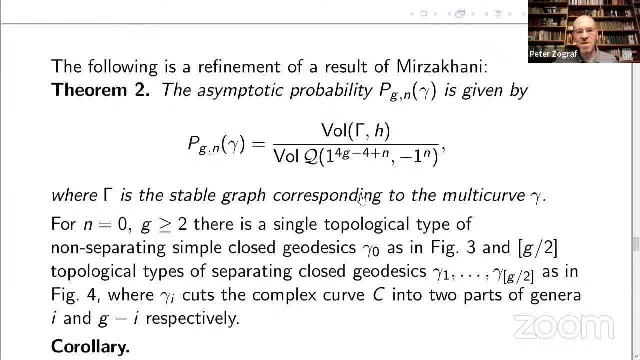 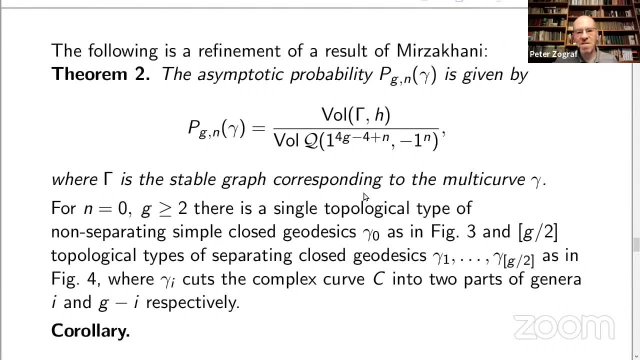 simple closed curves, closed geodesics, gamma 0, as in figure 3, and the integer part of g over 2, topological types of separation and gamma 0, as in figure 3.. For n equal 0 and g is greater or equal to 2, there is a single topological type of non-separating. 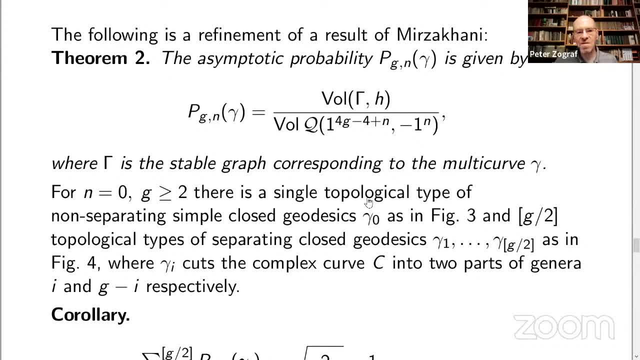 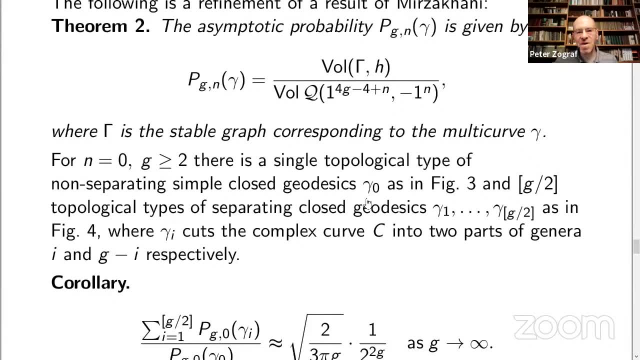 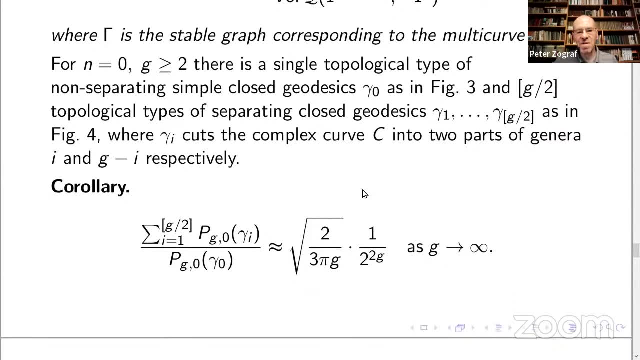 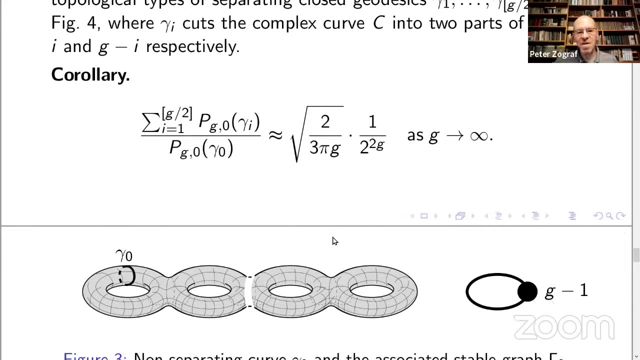 simple closed curves, closed geodesics, gamma 0. as in figure 3, and the integer part of g over 2.. As in figure 4, where gamma i cuts the complex curve into parts of general i and g minus i respectively. So let me show the pictures. So on the left there is a complex curve with non-separating 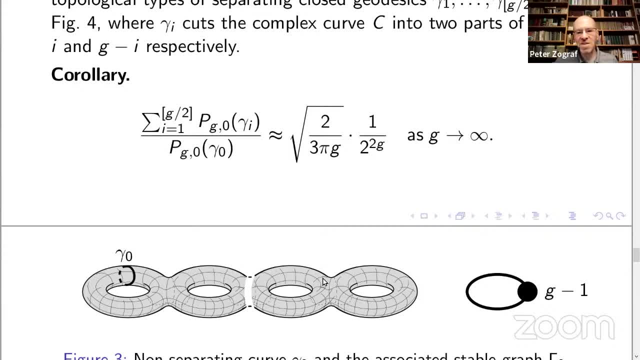 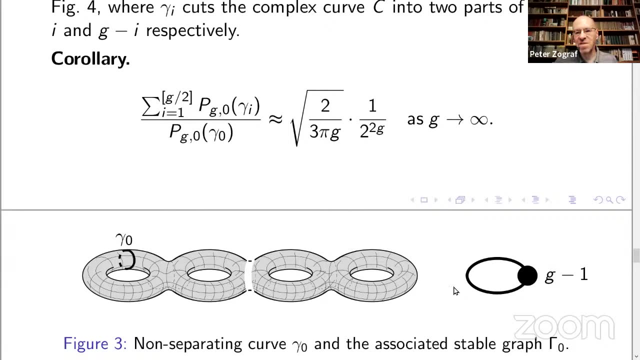 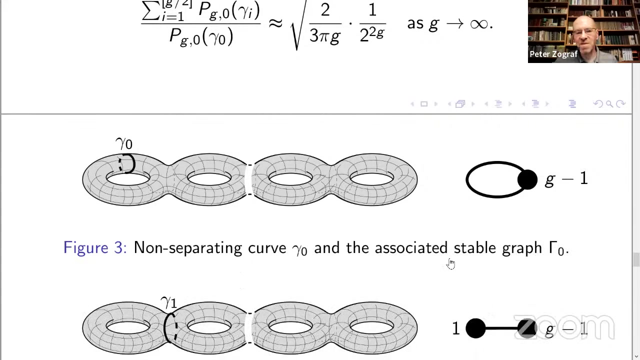 curves gamma 0, and on the right there is a corresponding stable graph. So it has one vertex, one edge, and the vertex is labeled by g minus 1.. That's the non-separating curve, and for separating curve we have 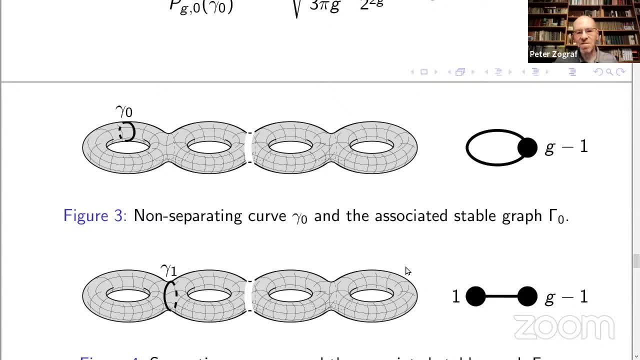 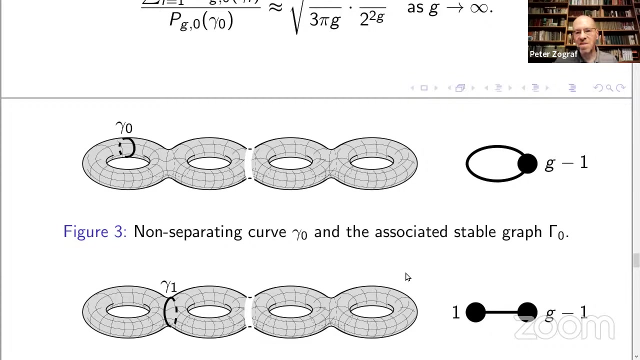 on the left the picture of a complex curve with a separating closed geodesic and on the right the corresponding stable graph. It has two vertices and one edge. Vertices are labeled by numbers 1 and g minus 1.. So these stable graphs are quite simple and it's possible to compute their contribution to the 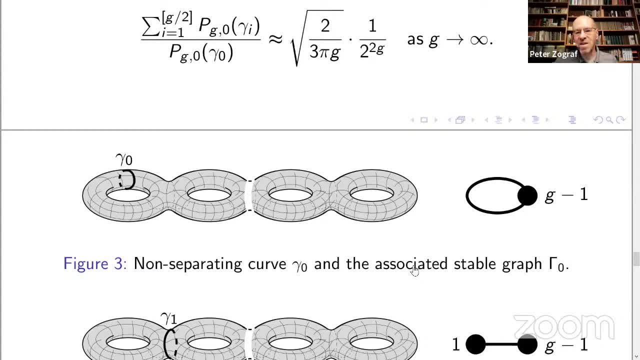 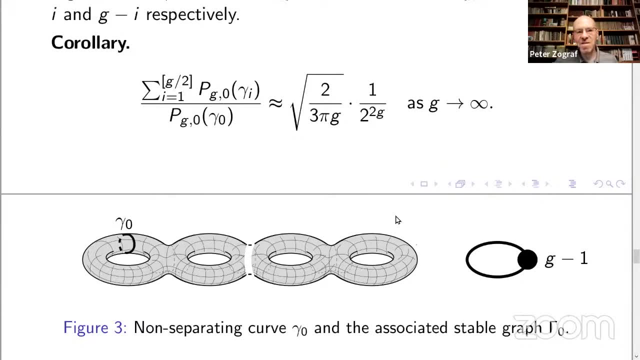 volume scale. So, for example, i drive by g minus 1, and the radius of height is the distance of a cap sprouted from an edge on g film. But the only problem is that our new Yes or No graph attaches itself to a deleted sel. There is p1, away from us. 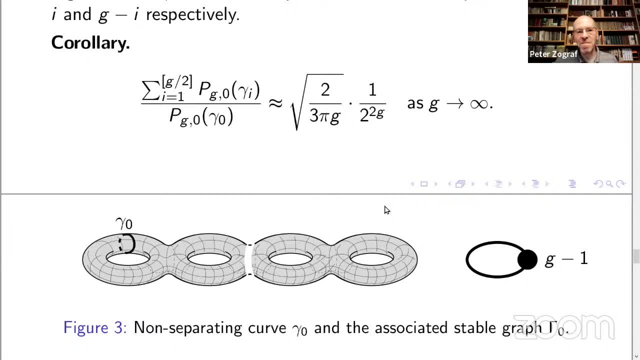 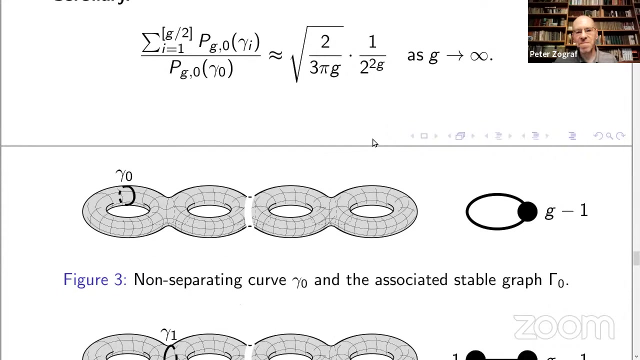 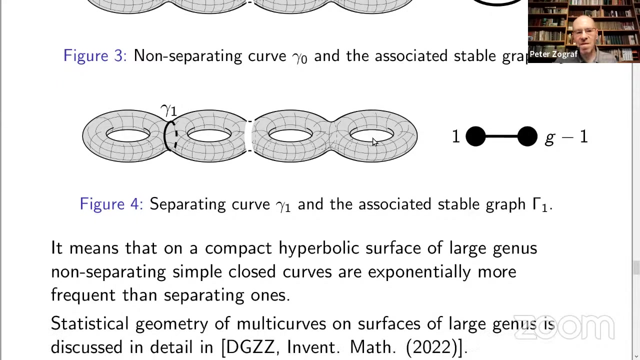 a complex curve over the probability that this geodesic does not separate curve is given by this expression. So we see that for large G the probability that the random closed geodesic is non-separating is exponentially more frequent than separating ones. 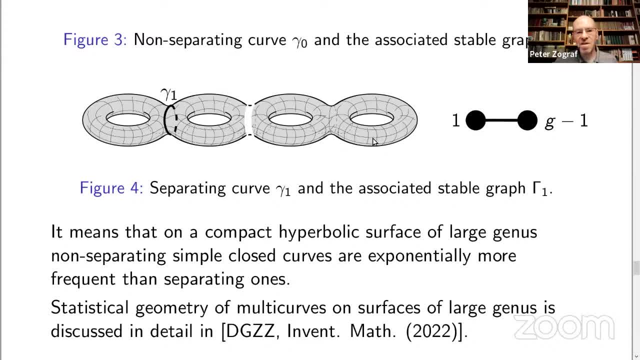 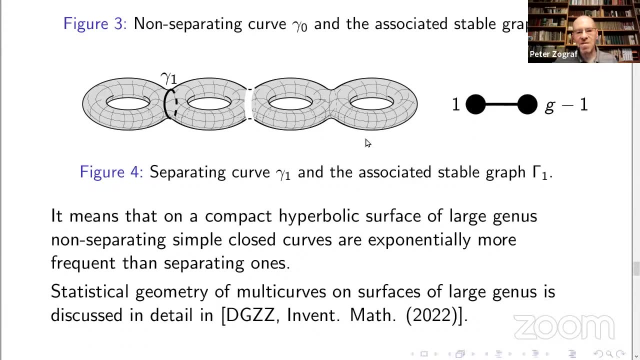 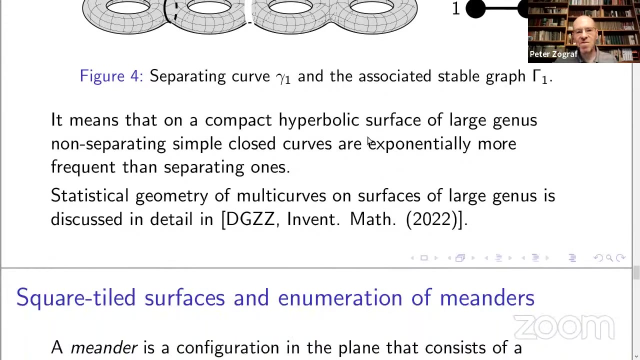 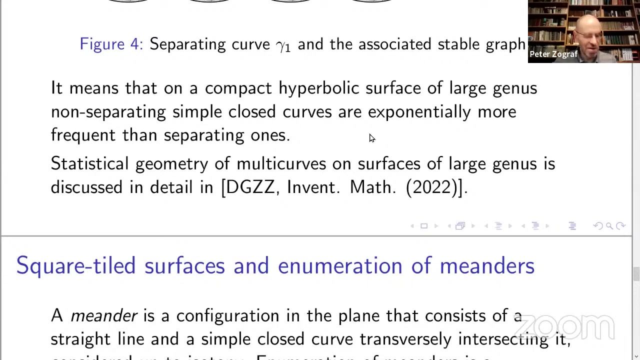 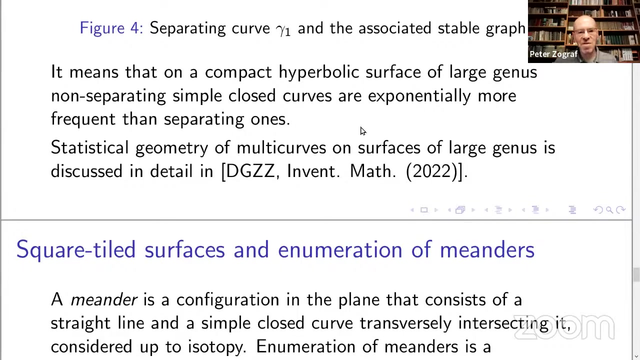 I would also like to say that this result was generalized to a small multi-curves on large genus, and it's discussed in detail in our paper with Delacroix, Gouchard and Soros. Now let's go to the third application of the latest point count, namely to the 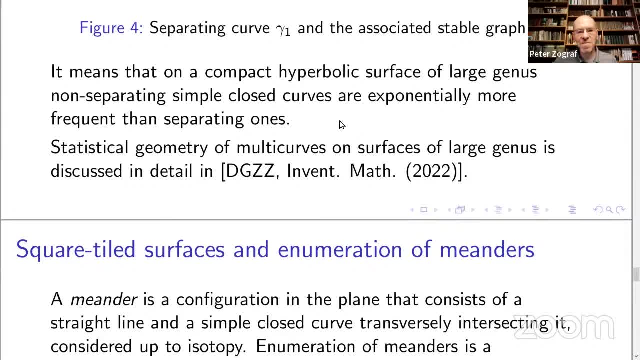 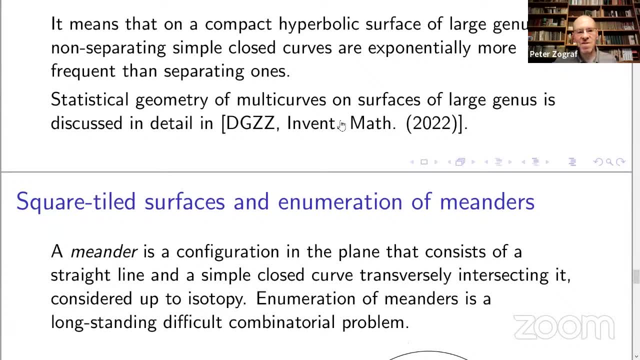 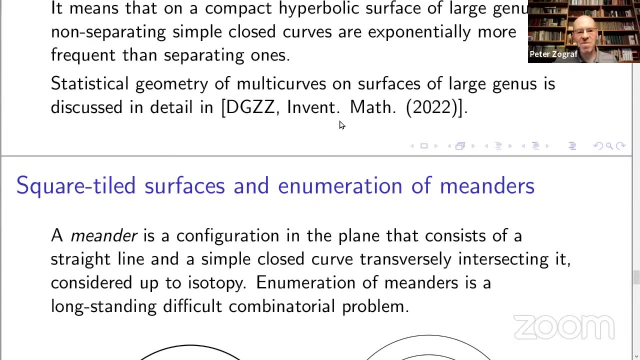 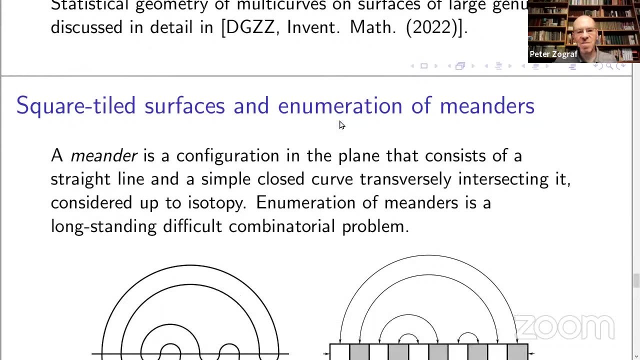 enumeration of meanders. A meander is a configuration of a plane that consists of a straight line and a simple closed curve transversely intersecting it. considered up to a isotopy. Enumeration of meanders is a long-standing, difficult combinatorial problem. 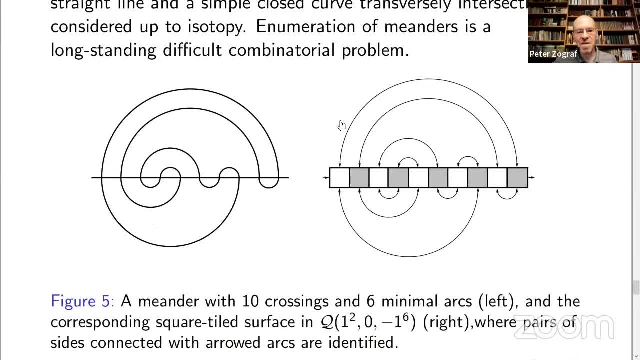 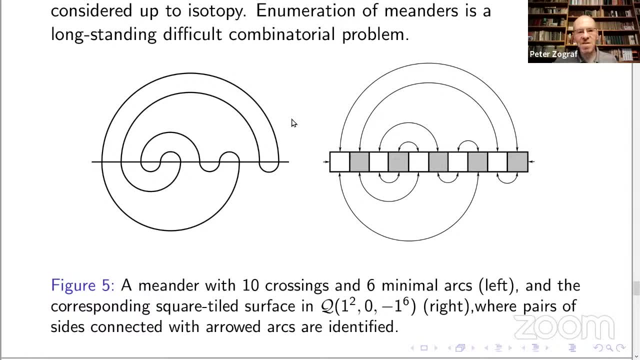 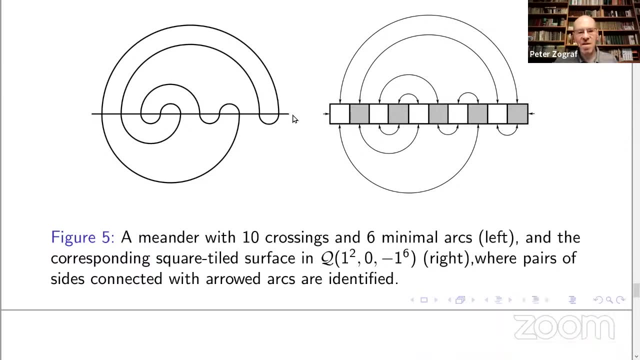 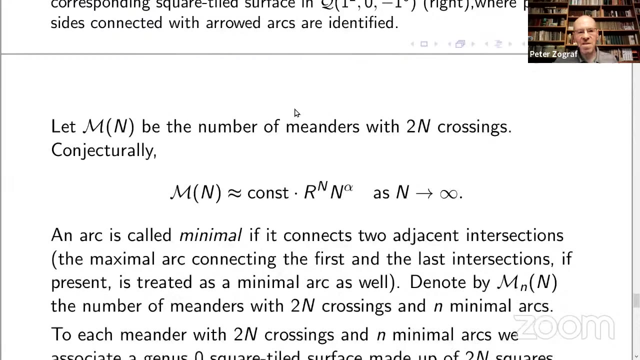 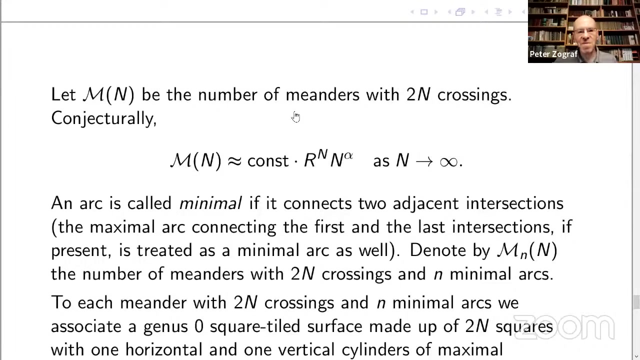 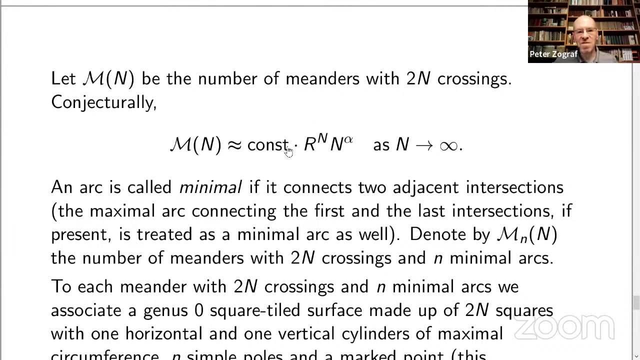 So here on this picture on the left, you can see a meander with ten crossings. Let M be the number of meanders with two N crossings. Conjecturally, this number behaves like an enumeration of a plane waves like this: It's up to some constant. It has an exponential factor r to the n. 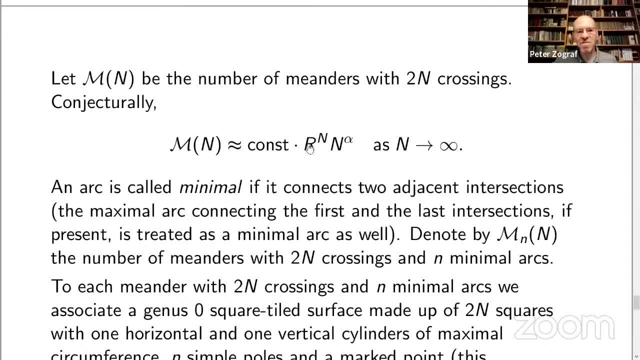 and polynomial factor m to the alpha, as n tends to infinity. So what is known? These numbers m of l were computed up to n, equal to 28,, I think. But there is a plausible prediction for the power alpha: that comes from interpreting the meanders as a. 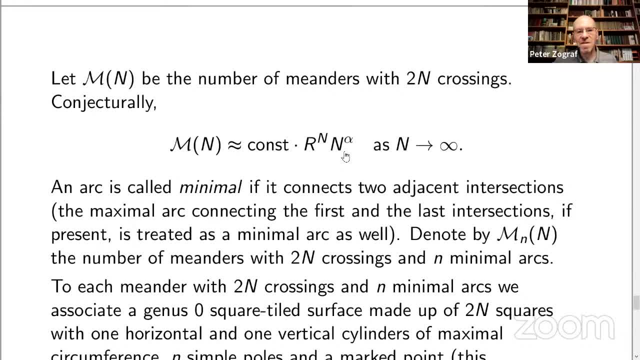 conformal field theory. That is due to DeFrancesco and co-authors, But there is no guess, even on the conjectural level. what is this number r? So there are not. so much is known about how this works. This number of meanders behaves for a large time. The situation becomes more tractable. 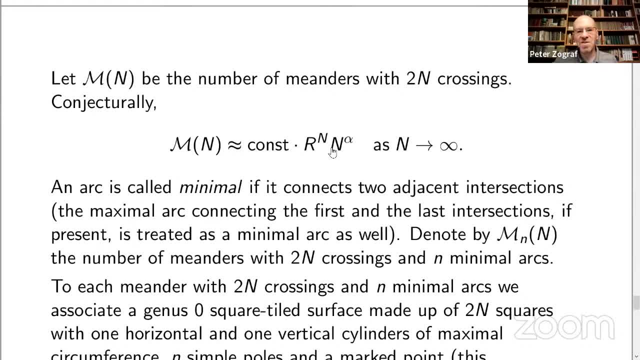 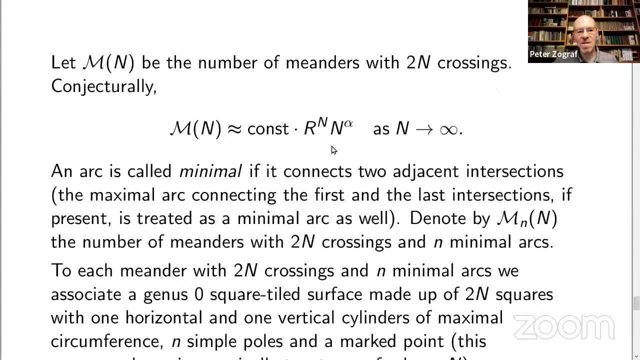 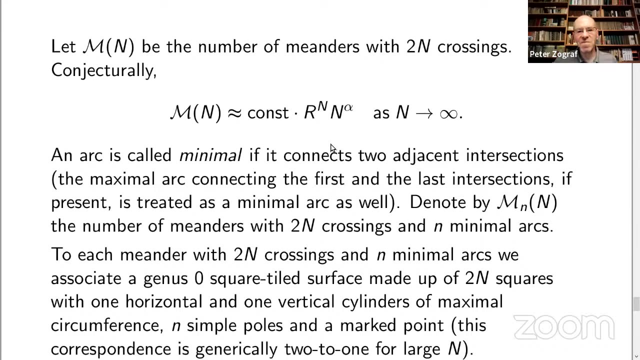 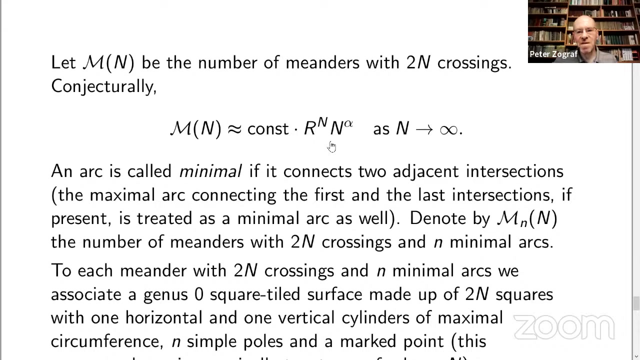 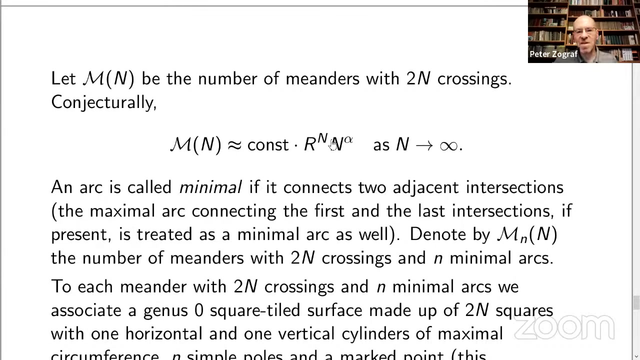 if one imposes additional topological conditions. An arc is called minimal if it connects two adjacent intersections of a meander. The maximal arc connecting the first and the last intersection, the present, is treated as a minimal arc as well. It's known by m sub n of m big the number of meanders, that's two n crossings, and 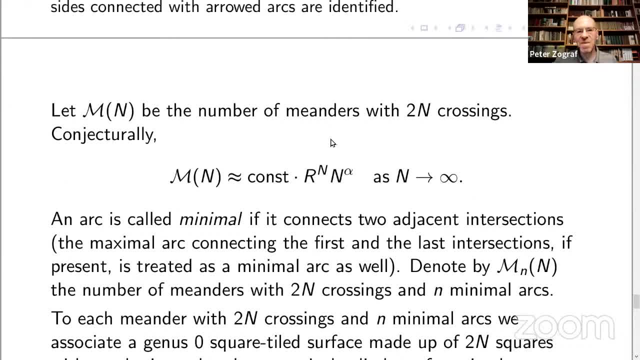 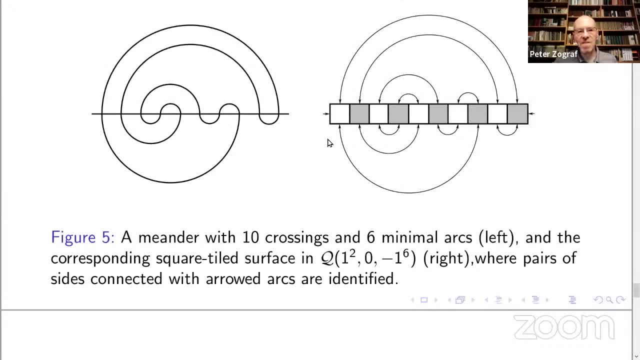 n minimal arcs. So let's go back to the picture. So on the left there is a meander with six, with ten crossings and six minimal arcs. There are five of them that are one, two, three, four, five minimal arcs that are finite. 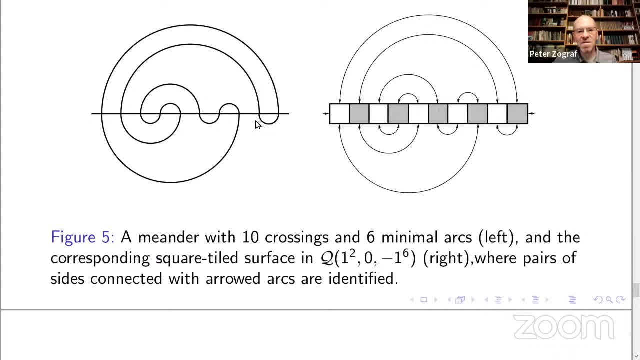 And then there is a meander with six minimal arcs. There are five of them that are finite. And then there is a meander with six minimal arcs- There are five of them that are finite, And there is one minimal arc at infinity. 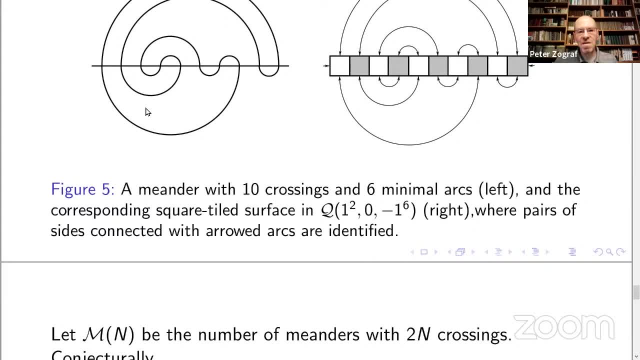 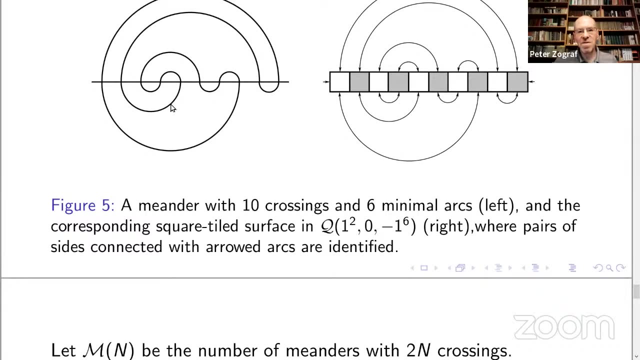 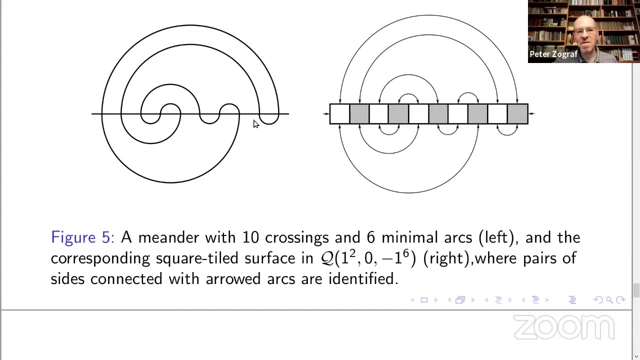 And that's the arc number six. And there is one minimal arc at infinity. So that's arc number six. And it's hard not to see that the meanders correspond to certain square-tile surfaces. So on the right you see a square-tile surface. 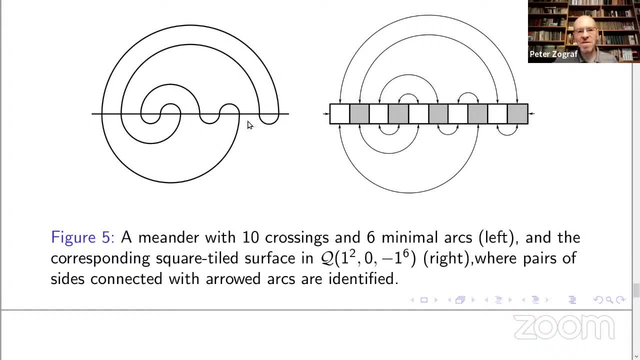 that corresponds to the meander at the left. The meander is for a regular graph, so what we have on the right is a dual graph to the meander and the arcs with arrows they show which pairs of sides are glued together. 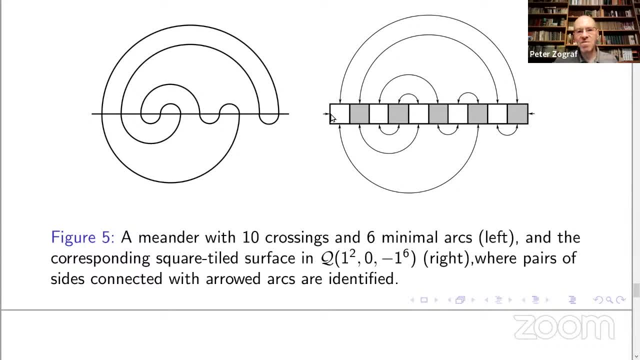 This square-tile surface is very special in the sense that there is only one horizontal cylinder of height 1 and maximum circumference, and if we make all the gluings, we can see that there is also precisely one vertical cylinder of height 1.. 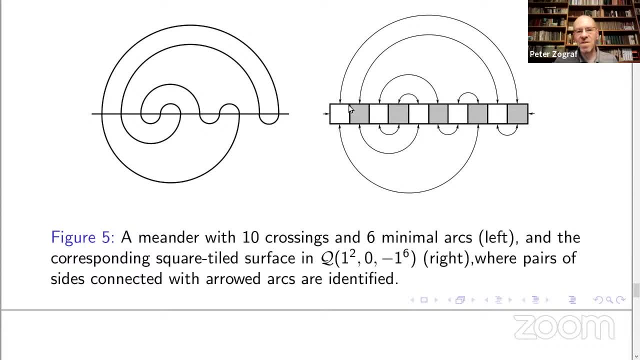 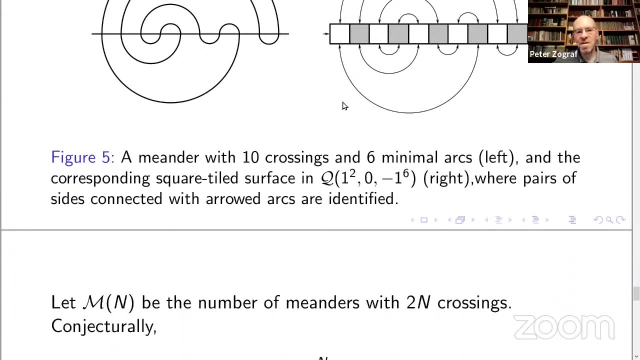 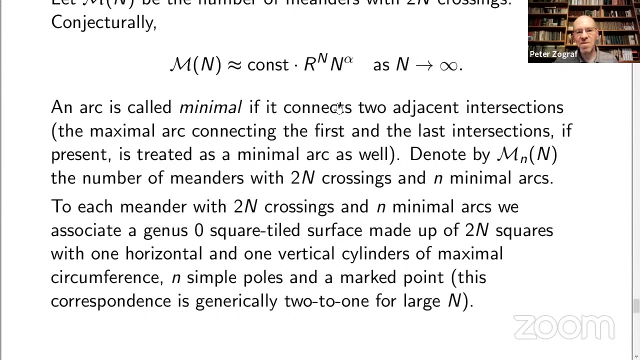 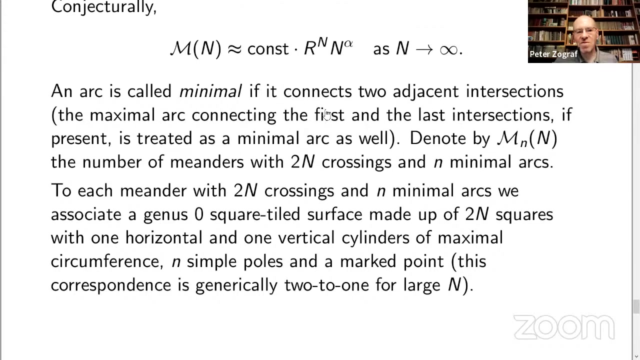 So we have width 1 and circumference maximum, circumference 2n. So there is correspondence to each meander with 2n crossings and then minimal arcs. we associate the genus 0 square-tile surface made up of 2n squares with one horizontal. 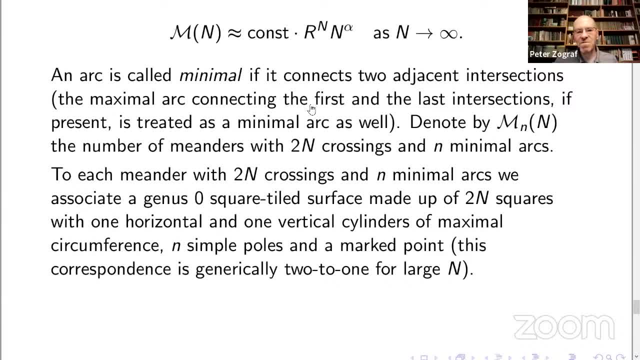 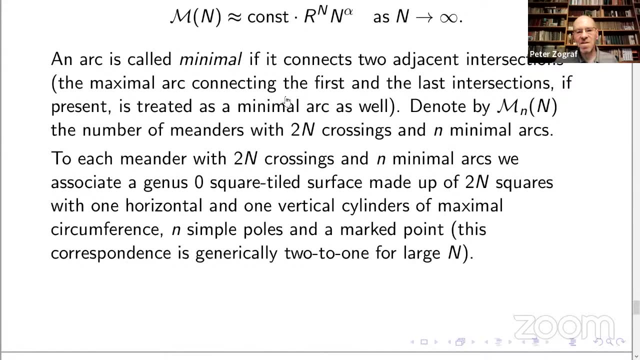 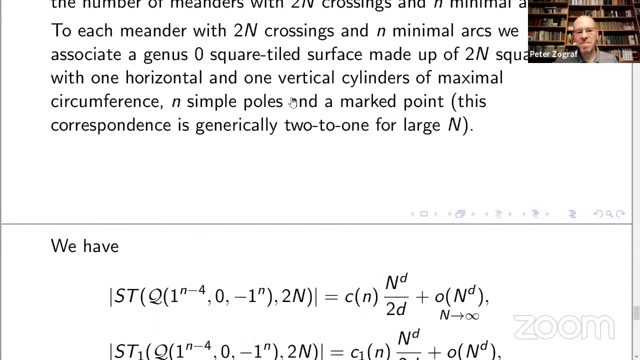 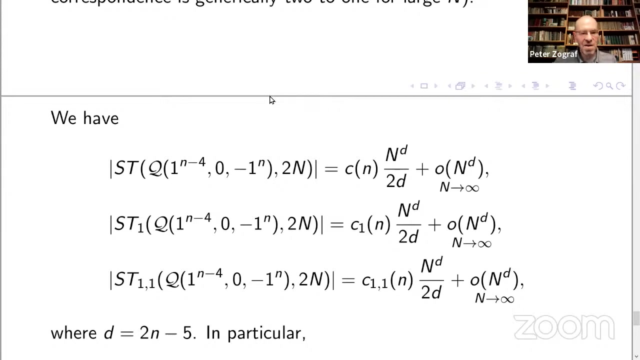 and one vertical cylinders of maximum circumference with n simple poles and the marked point. We need now to mark a point that corresponds to the point at infinity of a meander, and this correspondence is generically 2 to 1 for large n. So now let's consider three nested sets of square-tile surfaces. 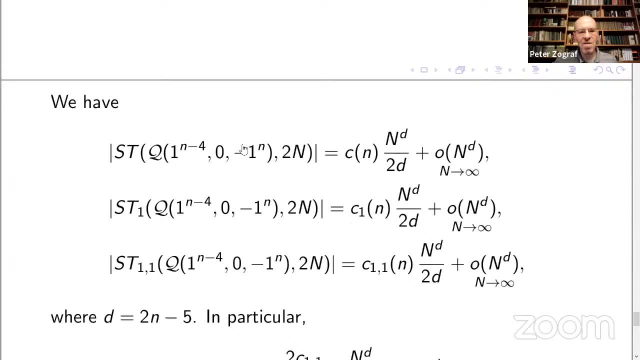 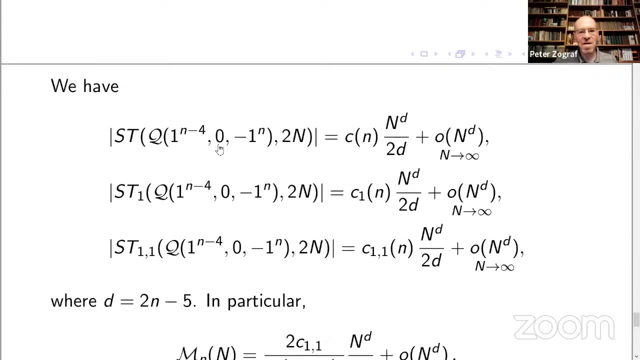 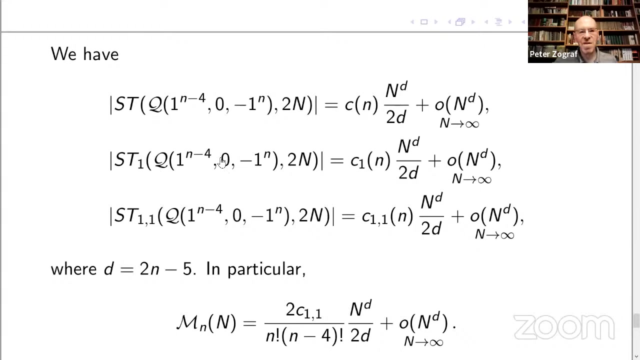 One is the set of all square-tile surfaces in the principal stratum, built of no more than 2n squares. The second one is the set of all square-tile surfaces with precisely one horizontal cylinder of maximum circumference width of not more than 2n squares. 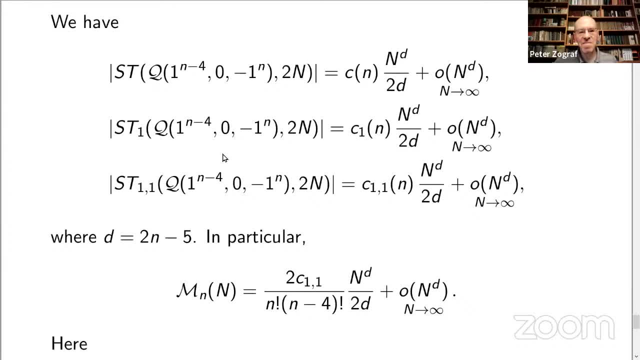 and the last set is the set of all square-tile surfaces in the set of square-tile surfaces, with one horizontal and one vertical cylinders, again built of no more than 2n squares. So these cardinalities of these sets behave like this: 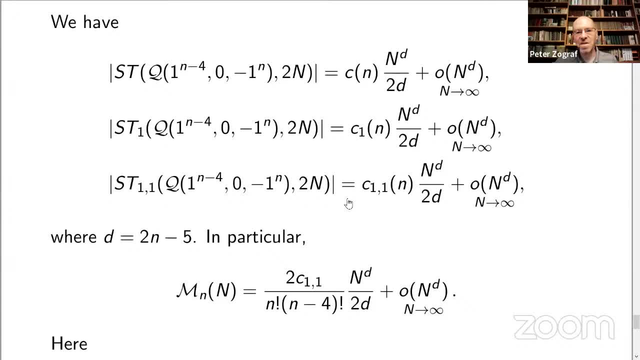 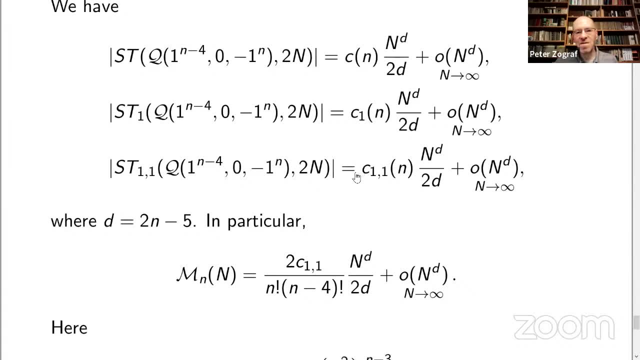 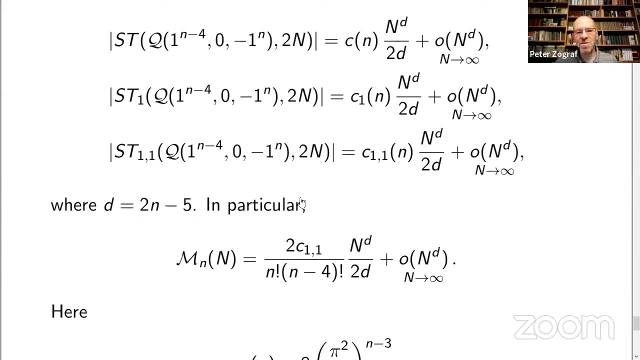 It's a square-tile surface given by these three formulas. Here d is the dimension of the modular space of quadratic differentials and in particular we have the following formulas. The following formula for the number of meanders with two n-crossings and n-minimal arcs: 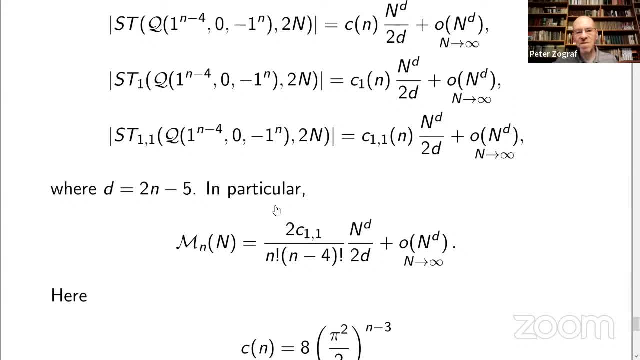 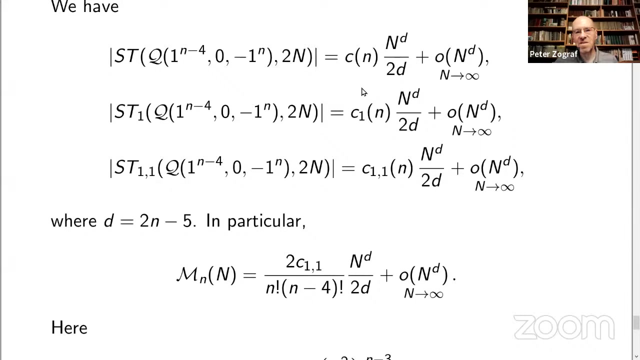 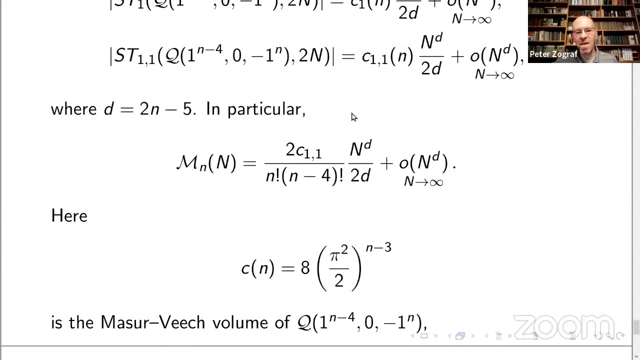 This asymptotic is given essentially by the constant c11.. We cannot access this constant directly, but we can do that in an indirect way. We can evaluate the constant c of n and c1 of n. c of n is just the major reach volume of the principal stratum. 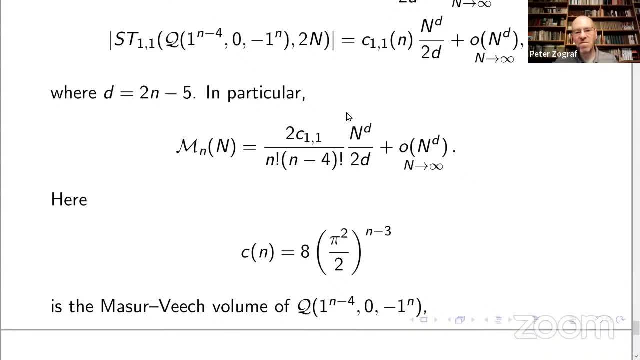 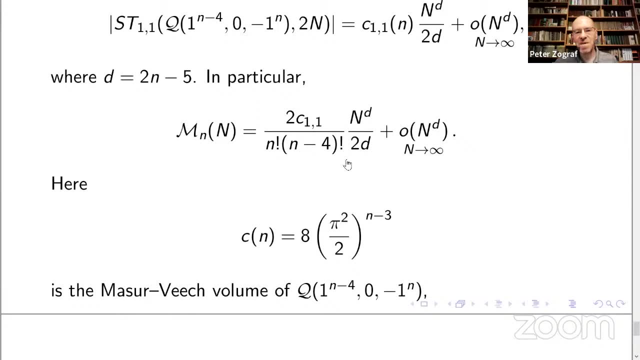 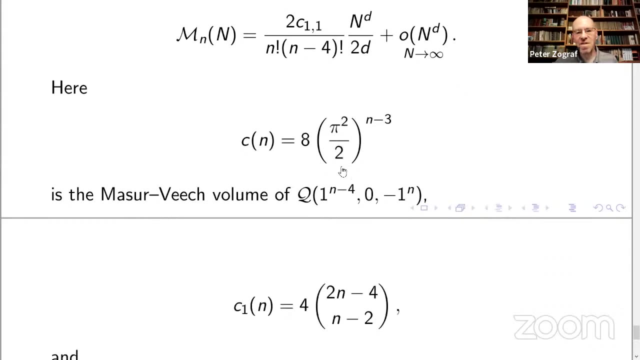 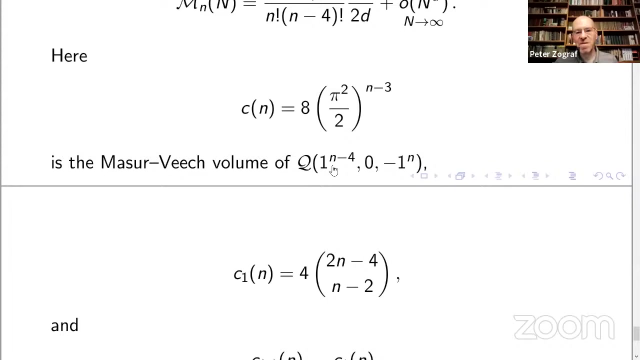 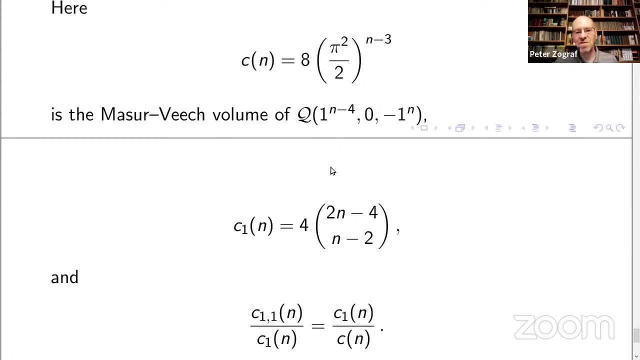 in the space of quadratic differentials of genome zero and n-simple poles. This formula was obtained by Atreya, Eskin and Zorin. The coefficient c1 of n can be computed by direct combinatorial consideration and it's just a binomial coefficient. 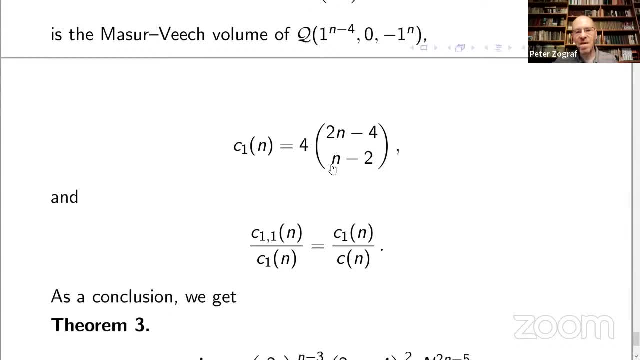 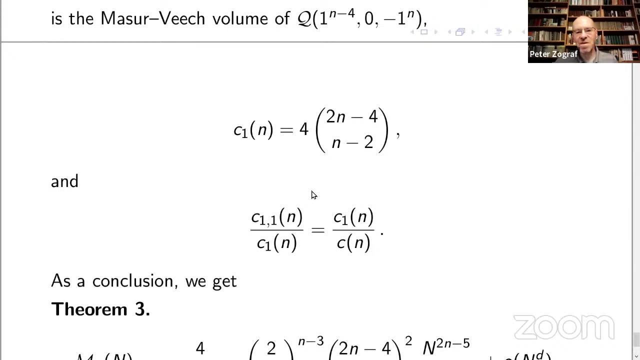 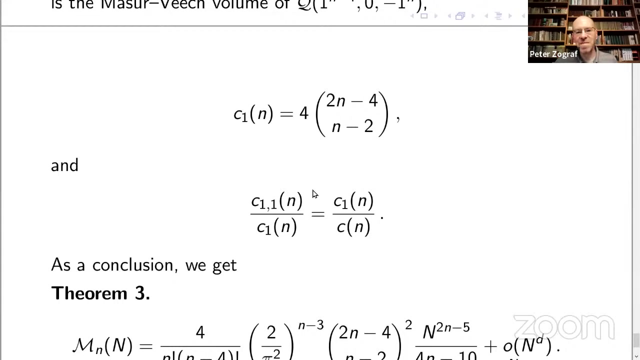 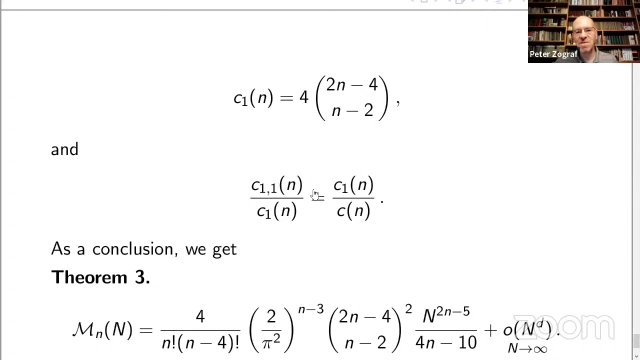 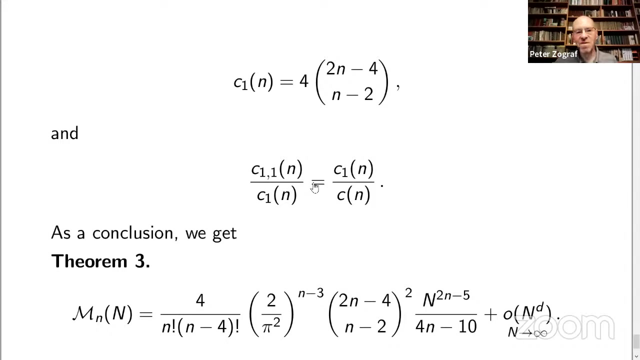 And at last, these two ratios, c11 over c1 and c1 over c, are equal. That follows from the fact that the numbers of horizontal and vertical cylinders, the horizontal and vertical decompositions, are asymptotically independent. As a conclusion of this formula, 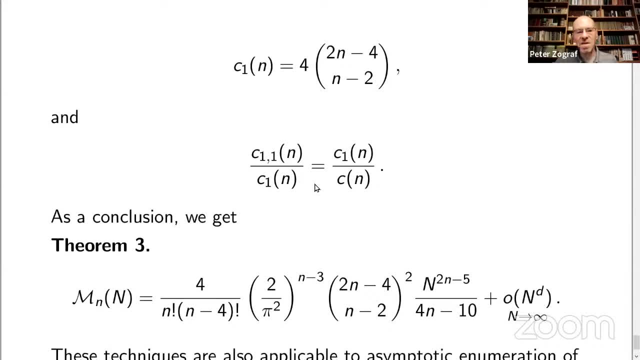 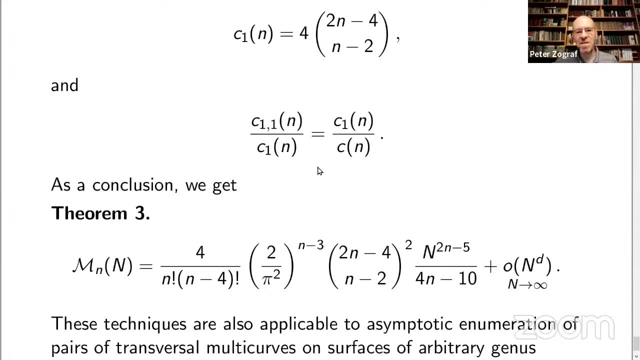 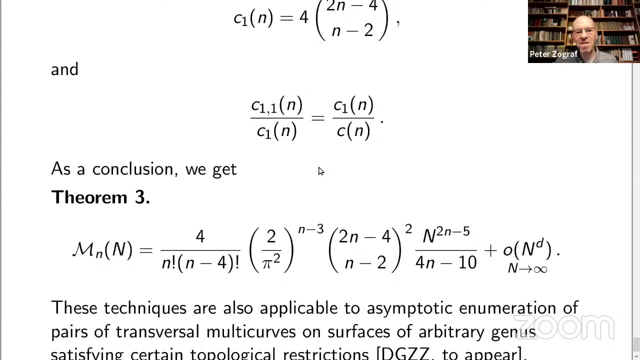 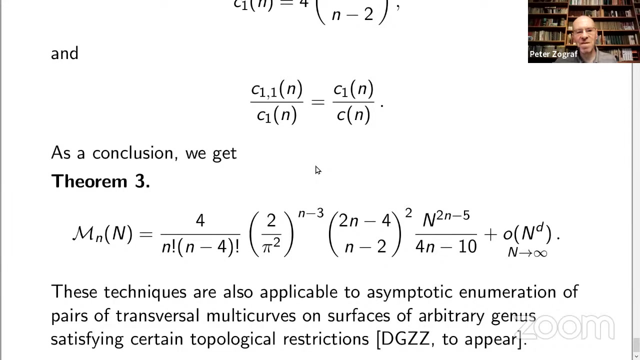 we get the following statement: We just express c11 as c1 squared over cn and substitute the formulas for them And we get the following expression for the number of meanders with the given, with the fixed number of minimal arcs, That is. 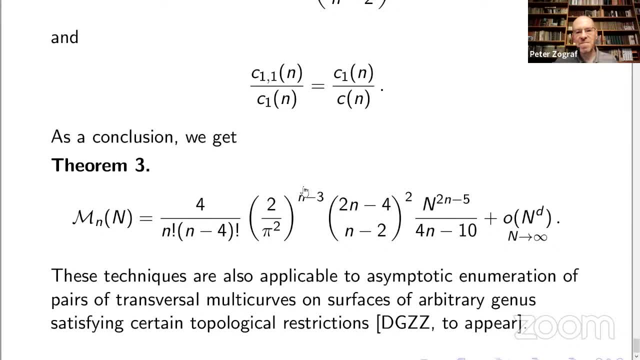 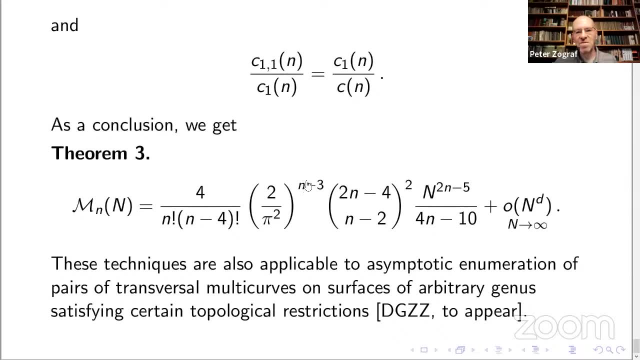 c1- Mob, c1, 0, 4, x, p, y … 4 0 100 d. So these techniques are also applicable to asymptotic enumeration of pairs of transversal multicares on surfaces of arbitrary regimes satisfying certain topological restrictions. 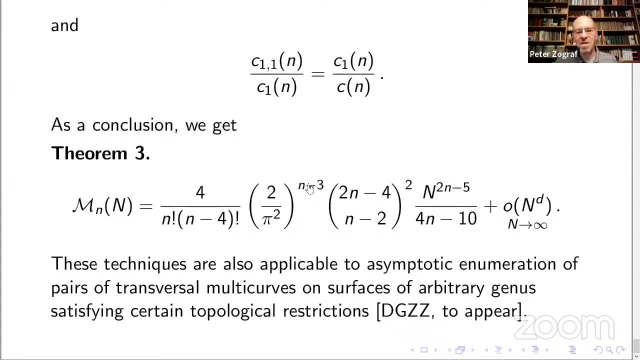 And that is the terminal joint paper with Delacroix, Gougin and Sorge. So here I'll stop. Thank you for your attention. Thank you for your lecture. We do not have time for, or it's not possible to, ask questions. 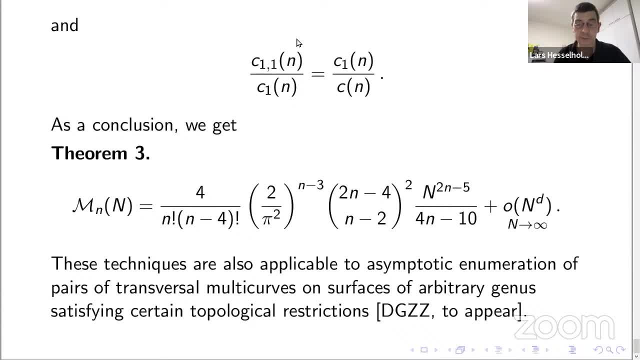 here, But if somebody has questions, please e-mail.